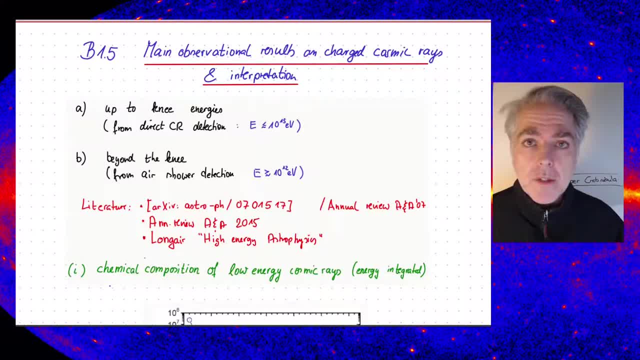 in 2007 and in 2015.. The paper in 2007 is also available through this archive number which I present here, whereas the 2015 paper is unfortunately behind the paywall. so if you want to access it, you need to be connected to a university domain, And then I also list here the paper, not the paper. 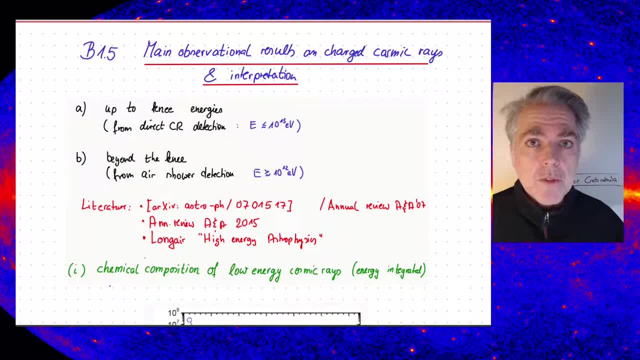 but the textbook, This book by Malcolm Longair, High Energy Astrophysics, where some of the discussions that I have here are actually done in a very similar way. So let's start out with the chemical composition. We had seen already in a previous section, where we discussed the main characteristics of cosmic. 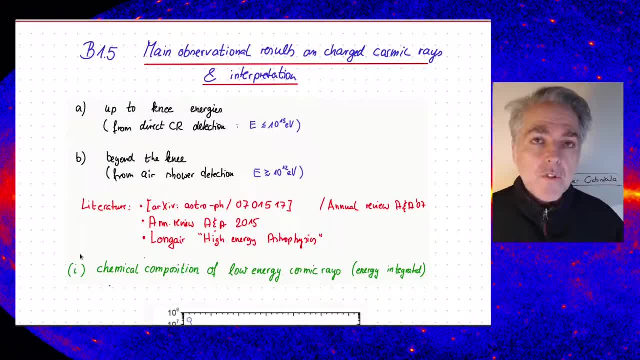 rays that, roughly speaking, the cosmic ray composition follows the composition of the interstellar medium, that is, the gaseous material that is between the stellar systems in the galactic plane, And that material is made up mainly of hydrogen and hydrogen and hydrogen. 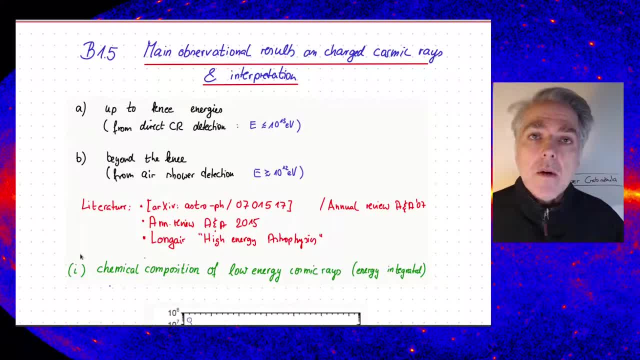 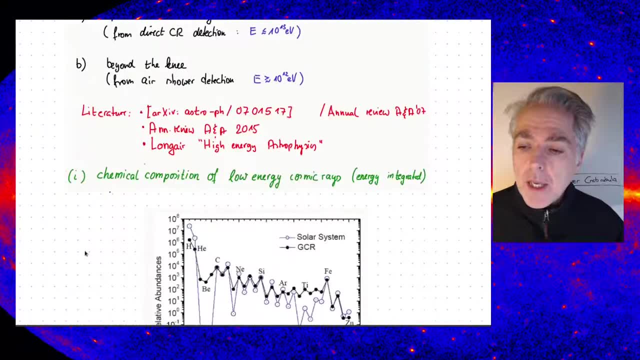 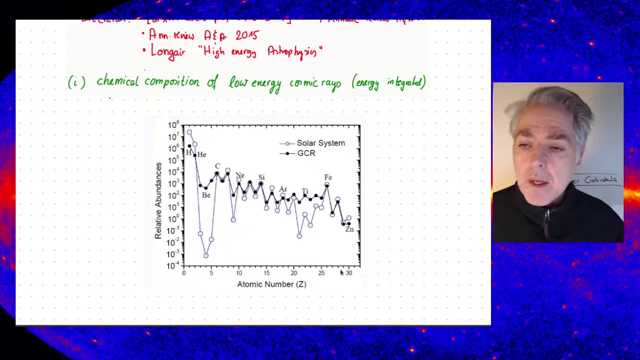 and helium and heavy elements which are produced in the stellar cycle. Now what I show now here is a plot where we have the chemical composition as a function of the charge number and it's plotted in relative abundance, which is normalized as you can see here. 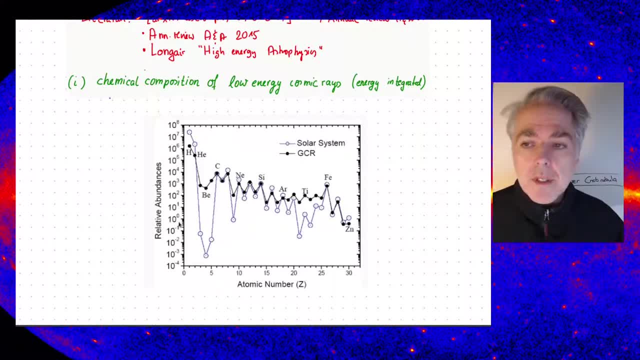 to some value of a heavy element. So it doesn't, this absolute scale doesn't really matter, it's just the relative abundance that really matters. And note that this scale on the y-axis goes over 12 orders of magnitude and the x-scale is just the charge number up to heavy elements. 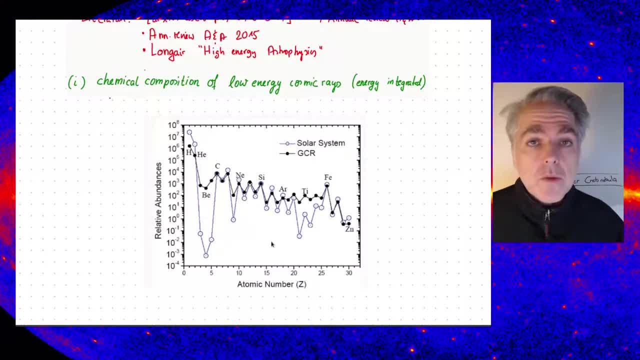 beyond iron, And there's two graphs. the blue one is the abundance that we measure typically in the vicinity of the solar system and the black one is the abundance that we measure in galactic or charged cosmic rays. This is energy integrated, so this goes for several hundred MeV or GeV energies in terms. 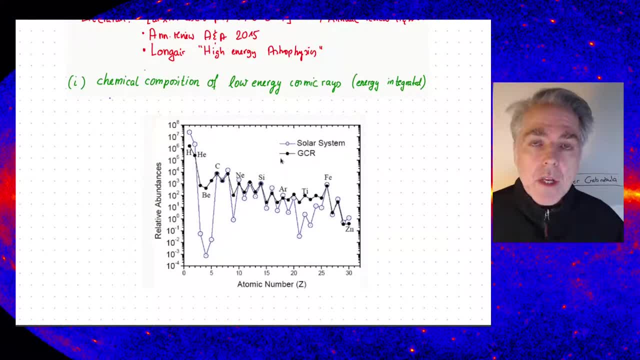 of kinetic energy, integrated up to high energies. So this is, if you think about it, not resolved over energy, but just integrated over energy, which is, of course, dominated by the low energy part of the cosmic ray energy spectrum. Now, if you compare the two graphs, you find that 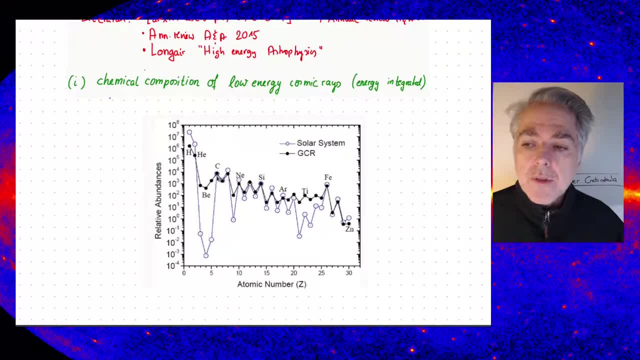 for many of the species, like, for example, carbon nitrogen and oxygen, the abundances are very, very similar. The abundance is very, very similar. The abundance is very, very similar And you find that the actual shape is very similar and also the relative abundance. 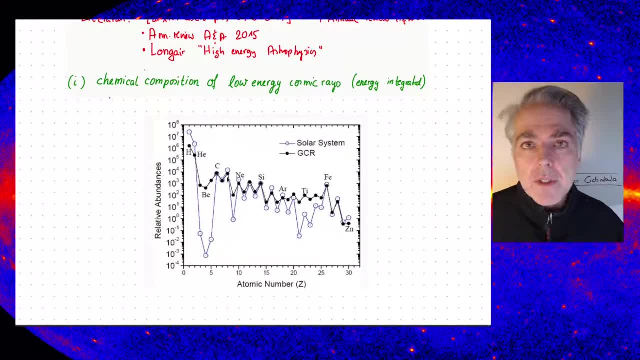 of these three species among each other is similar, just with a slight difference in the oxygen. You find that for most of the species up to just almost close to the iron, you will find also very similar numbers. So silicon is very similar, neon argon is very. 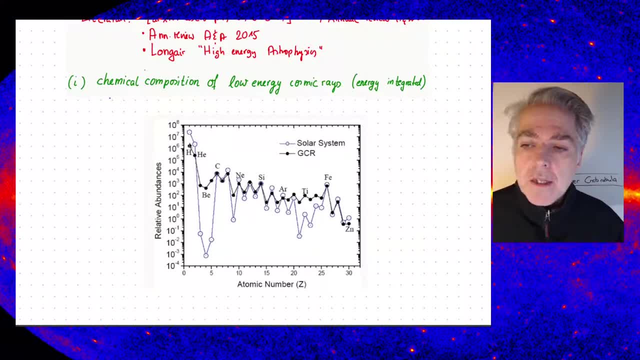 similar, and so on and so forth. You also find a similar shape in terms of helium and hydrogen, even though there's slightly less hydrogen, apparently, than helium. But if you shift these two curves, you basically will see that the relative abundance is about again the same. 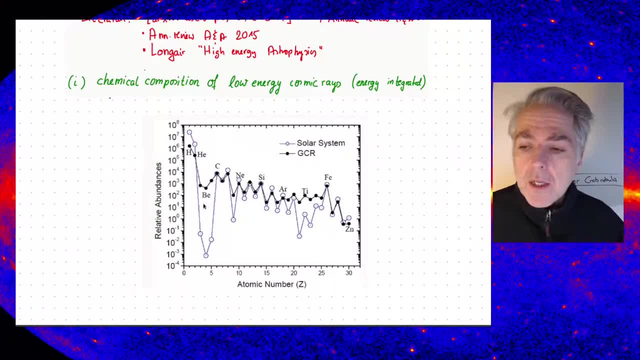 There's, however, also noteworthy differences. So if you look, for example, these three elements which are just short of the carbon, nitrogen and oxygen- so this is lithium, beryllium and boron- you find that these three species are very, very underabundant in the interstellar. 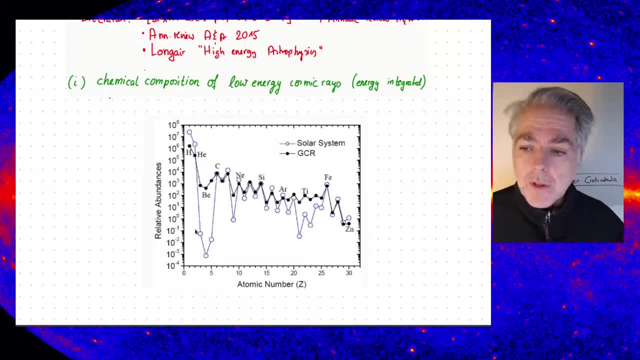 medium need this very huge ratio here. So if you look at it essentially, there's a difference between the relative abundance of lithium, beryllium and boron in galactic cosmic rays, which is of the order of almost 1 million times for beryllium, as an example. So that means that there's some mechanism. 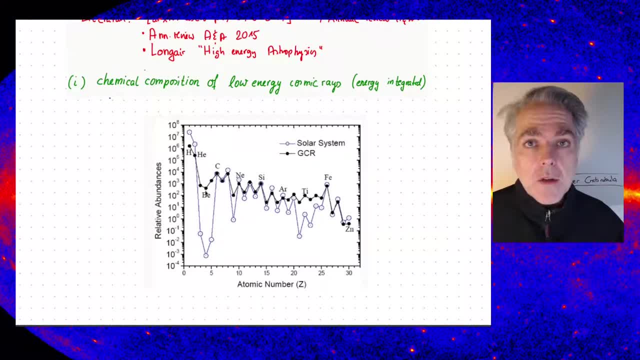 which produces somehow lithium, beryllium and boron in cosmic rays which are not present when the particles are being ejected, accelerated and become cosmic rays, Whereas the cosmic rays seem to be otherwise. following fairly much this interstellar medium abundance, You find also a similar type of feature, just shy of the iron. So this group here 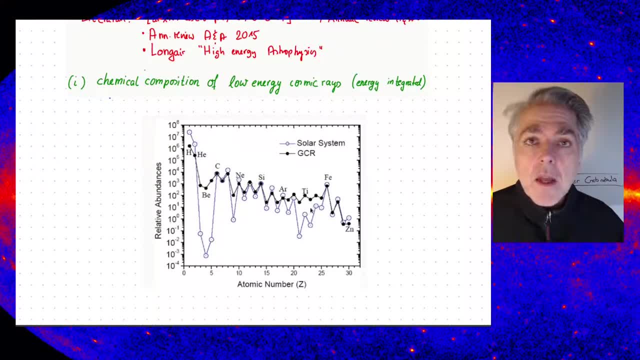 this is titanium, scandium and so on, which is also overabundant, not as dramatically as you notice here. this is just about a factor of 1000.. Then, in the case of lithium, beryllium, boron, so this light elements are produced. Now let's start discussing this in terms of what? 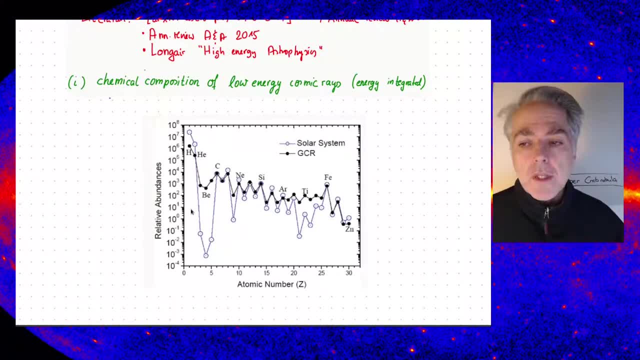 could be the origin of this. You could, of course, always assume that there's somehow an environment and where the cosmic rays are initially accelerated and injected to become cosmic rays, that this is somehow having a larger abundance of lithium, beryllium, boron, and it's present in the otherwise typical interstellar medium. 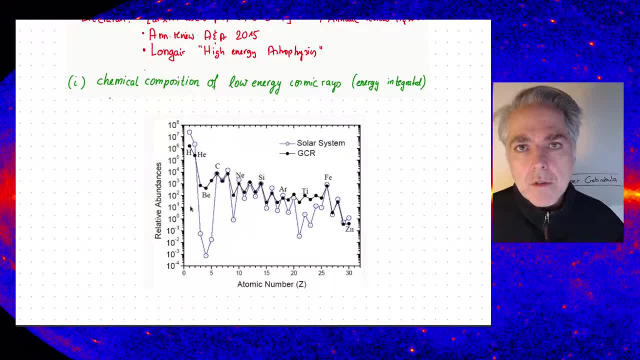 This seems a bit unlikely and difficult to understand, because these three elements have a low abundance for a good reason. The reason being is that they are usually not produced. in the stellar fusion cycles, Lithium, beryllium, boron are produced. 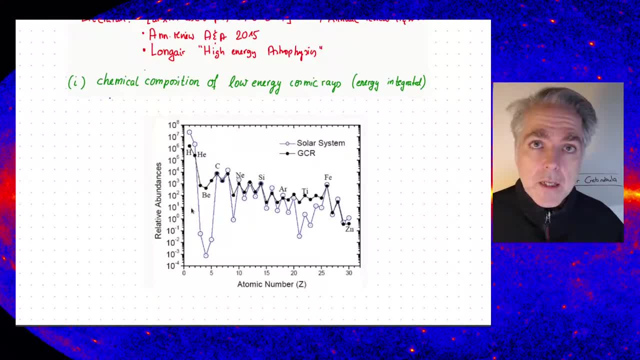 but they're also being used again for higher charge number species which are produced. So, roughly speaking, stars do not create lithium, beryllium, boron. The abundance that we measure here is pretty much the primordial one. That is, the one that was produced during the Big Bang. 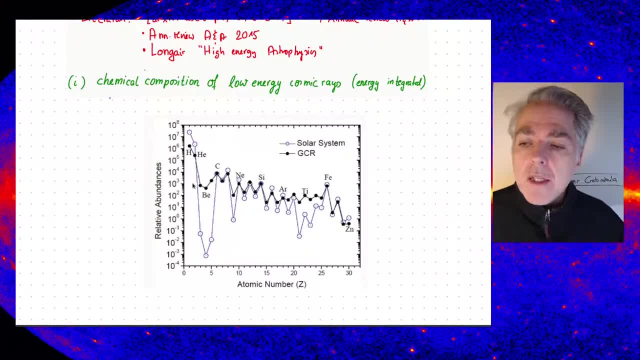 nuclear synthesis, which we will revisit later on. So there's no really easy source dependent relation for this overabundance. So there's, however, a much more natural explanation which basically gives us a very good description of this. So let's assume that you have carbon. 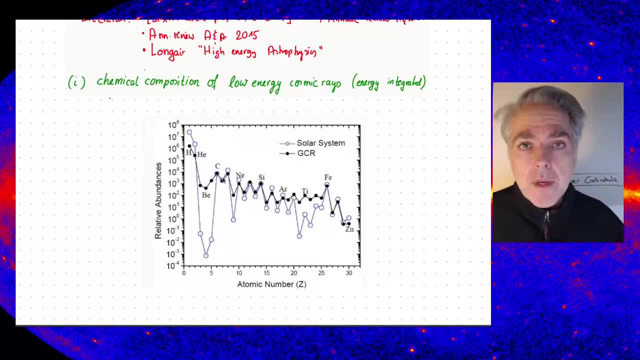 nitrogen oxygen interacting with the interstellar medium. So you have the relativistic carbon, for example, which will hit an inelastic or do an inelastic scattering process with the gas and therefore will then will then produce a residual remnant of the carbon which will be 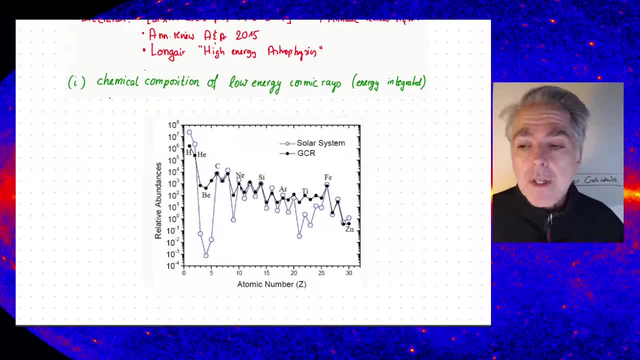 probably containing some fraction in lithium, beryllium and boron, The same with nitrogen and oxygen. So if you deplete a little bit of these three elements, you basically end up having, through spallation, a naturally produced overabundance of these. 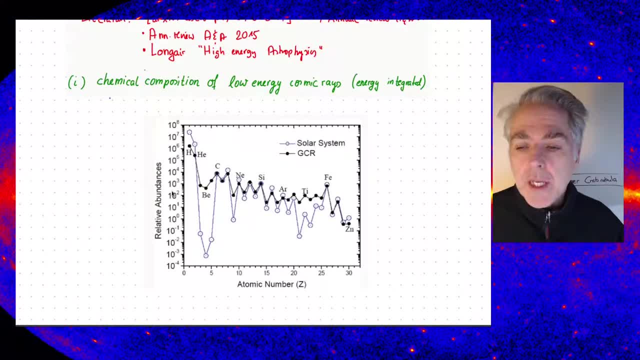 elements here. Let's do it a little bit more quantitatively, so we can do this in a very simple model. This simple model is oversimplified, So, mind you, this is not how we actually describe cosmic ray propagation in the galaxy. However, this gives us a good idea. 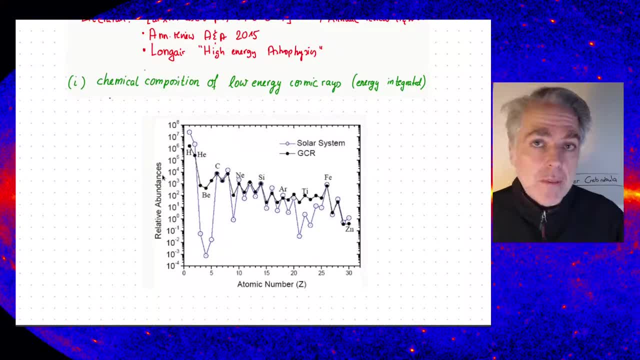 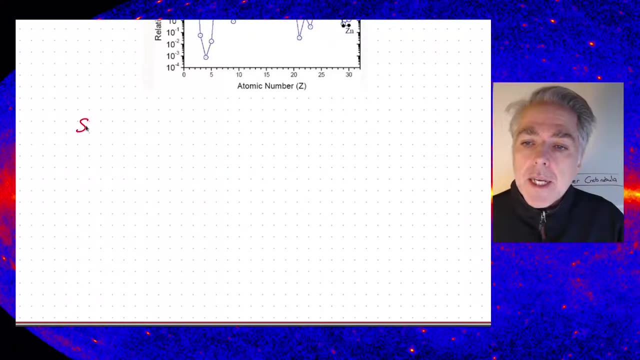 whether this assumption of spallation is or this hypothesis of spallation is a good one. So let's start out basically coming up with some hypothesis. So we say: spallation of cosmic rays produce lithium, beryllium and boron. 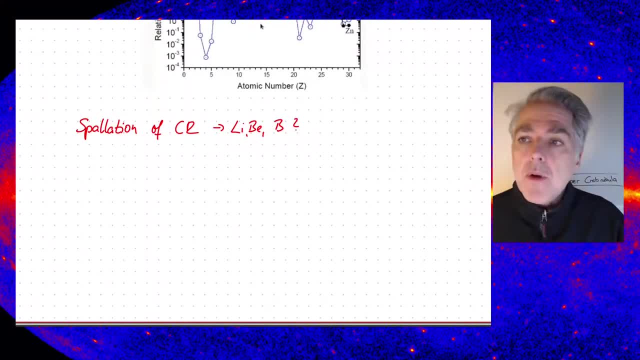 So that's our hypothesis, And the very simple model that we're going to do is just a so-called one slab model. So let's assume we make a very simple type of picture. So this is now some kind of- you know, homogeneous material which is between us, as the observer, and the sources. 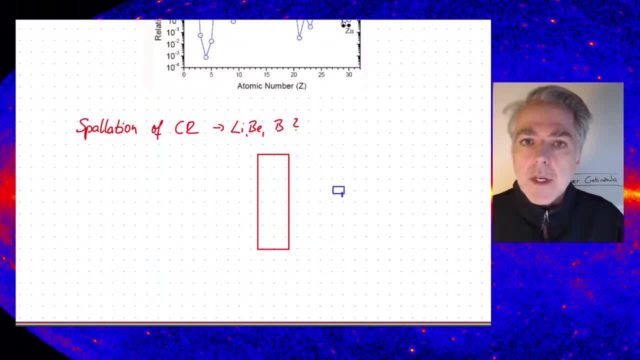 So let's store the source on the right side. Sorry, this has got to be the source on the left side. So this is the source and we are the observer on the other side of the slab. So the source will produce cosmic rays, They are being injected. 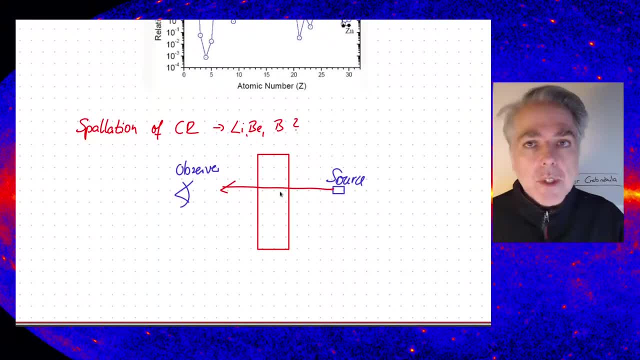 and so they pass through this one slab. So some of them will just basically pass through without any interaction, and some others they will interact here, So we'll have some interaction process here, and then you basically produce a very simple model. Let's assume now that 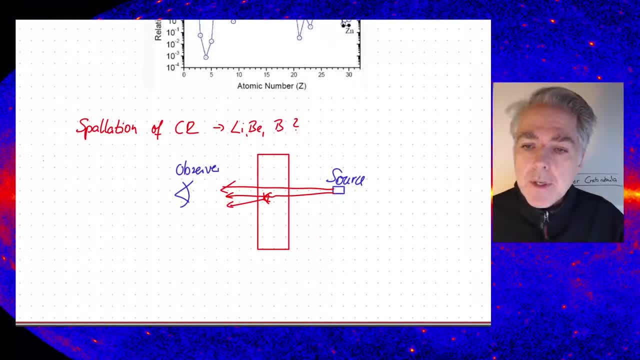 our, you know, this is a one slab model, That our one slab of matter is homogeneous, So we have a homogeneous density, So the mass density should be rho, And let's assume that the path length, so the distance through which the, the matter of the, 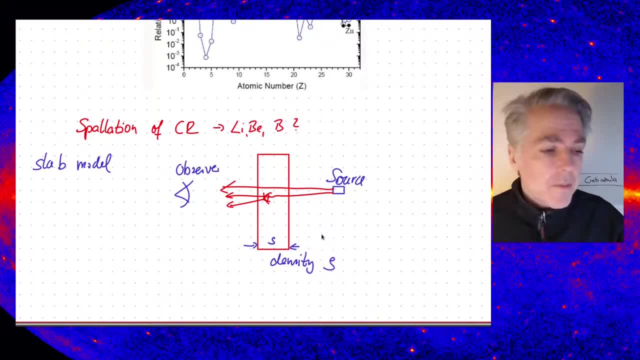 cosmic rays pass has a thickness of s, Then we can basically say that the xi value, which is the mass, the column density, is simply given by the integral ds times rho, And so this would be simply. the total distance of this thing will be s. 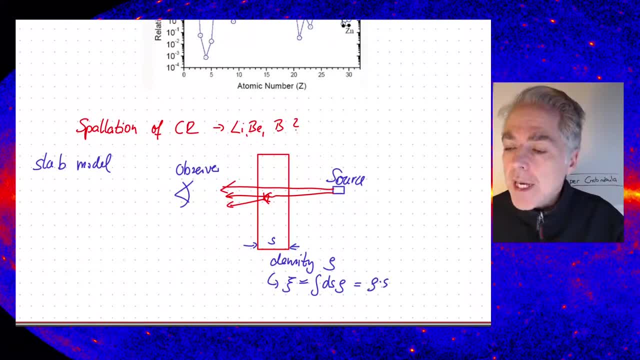 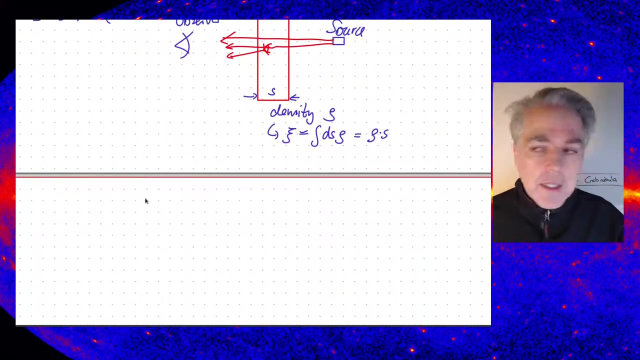 So we would basically say: this is then rho times s, And so that is something that we can assume, that it's homogeneous, And so we have just one number Attached to this one slab, And that's basically characterizing everything else. Now let's go on with a simple model. So how far can we? can we take this? 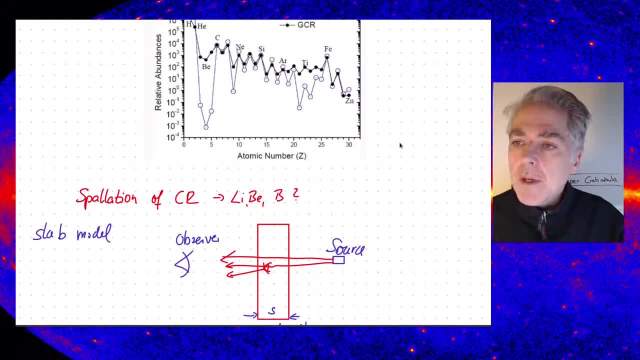 So let's assume now we are not going to be interested now in dealing separately with carbon, nitrogen, oxygen, And let's ignore everything beyond that, because they are subabundant. So basically, you see, for example, the next species which is abundant here is the neon. 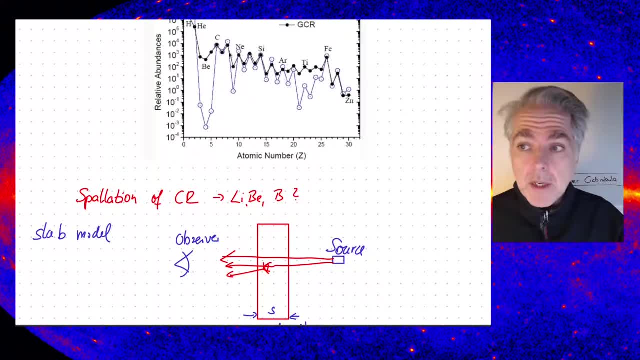 But that's already a factor 10 below each of these three c and o. So let's, let's put these three together, Let's make this this. no, sorry, this is a bit too much. Let's just make those three. Let's call that the medium group. 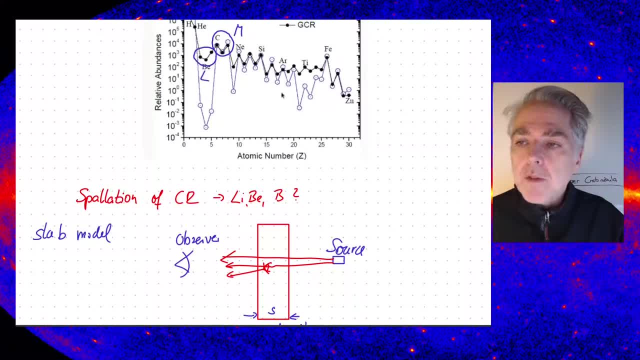 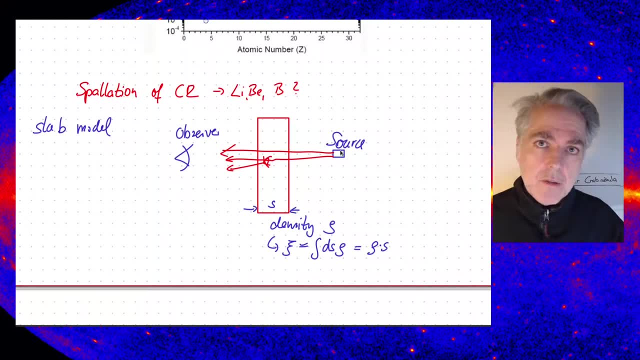 And this, these guys here, we call the the light particle group. So we make life a little bit simpler here. So let's assume we we do not have any light particles at the source. This is a good assumption, because if we look at the stellar medium we can say that at the source l 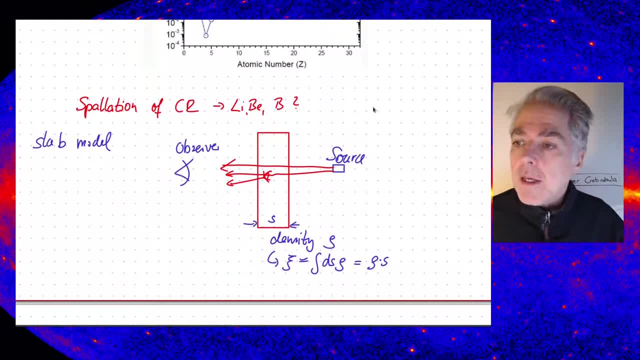 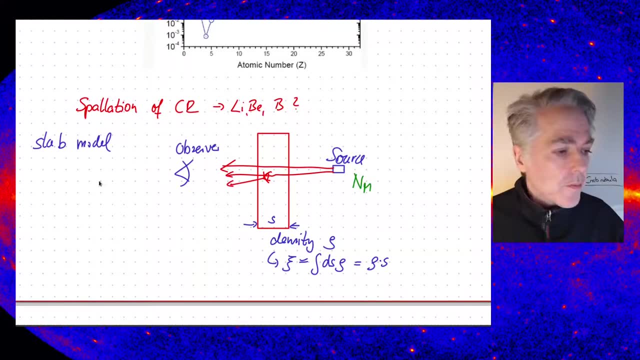 is essentially gone. So let's assume we have a number, density, nm, that we start out with, So that's produced and emitted by the source. Let's ask ourselves now what's going to be observable for us. So nm, as a matter of fact, should be then n carbon plus n oxygen plus n nitrogen. 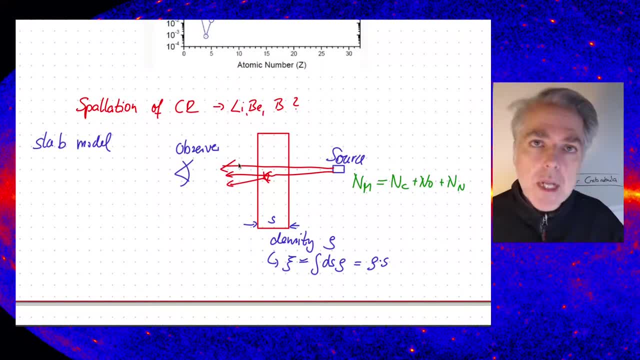 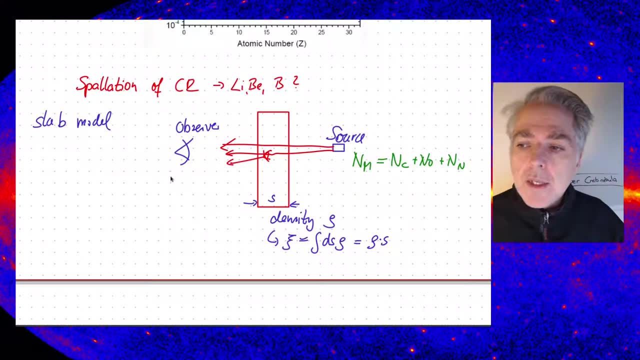 So n could be a density, it could be also absolute number, it doesn't really matter. Let's assume it's an absolute number of particles that we inject. So we will see then nm after xi and let's see how big that value is. And we would have then nl after after xi, to be then the sum of lithium, beryllium and more. 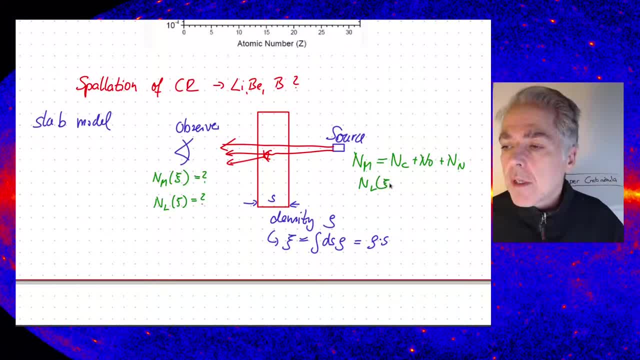 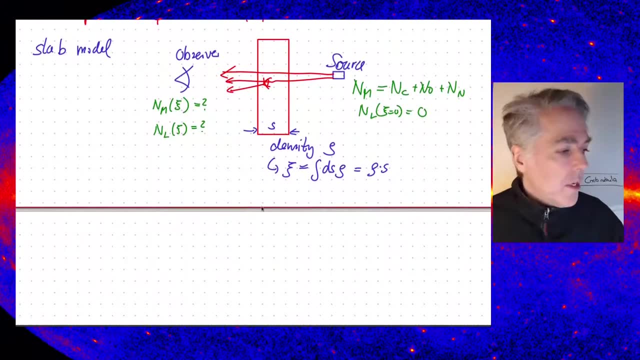 So let's assume nl for xi equals zero equals zero and m of is the one that we have in xi equals zero. So let's see we can make a very simple equation for this. So we can say the number of particles will change per path length. 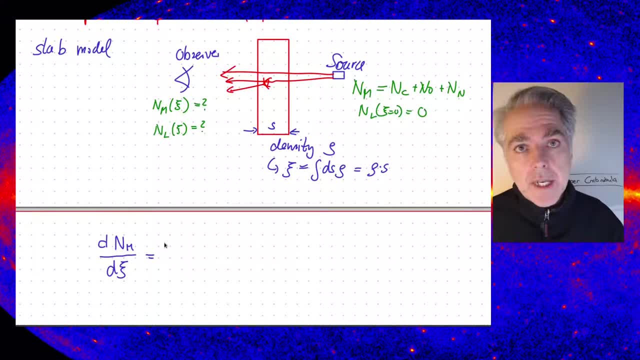 by assuming that there is an interaction length over which the interaction takes place. Let's call that xi m. So there will be a minus here because we will deplete the particles which have an interaction length of xi m. And this will be then. if it just this equation would be valid, it would be just an exponential 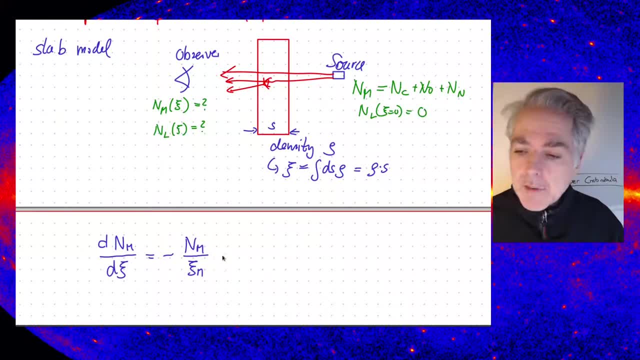 as a solution for this. However, we also have to take into account in principle, what we will neglect that in the following anyway, but let me just write down the term here- We will also have higher species, higher mass species, for example neon, silicon and so on. 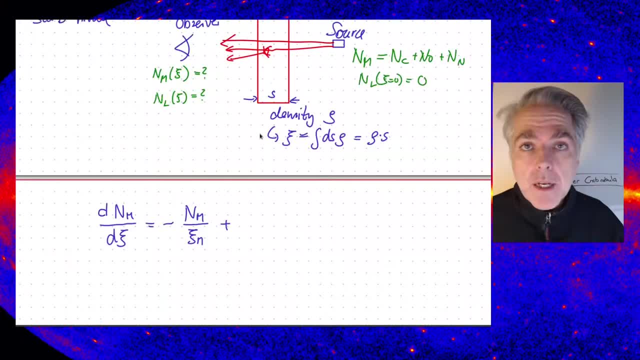 and so forth that would interact with the interstellar medium and they would produce this. so there would be additional particles coming nm, or particles of the medium group being produced through spallation of more heavier ones, And let me write that down so that would be, for example, the probability. 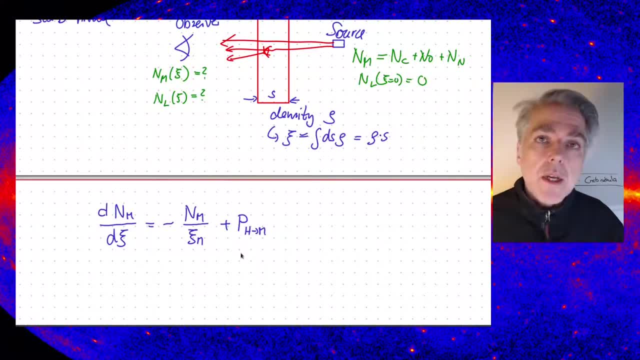 for a heavy nucleus to do spallation, to produce a nucleus of the medium mass range, And then we would have here the number of particles which are heavier than our medium mass group divided by the corresponding interaction length. xi, h, Now xi is related to the cross section. so the larger the cross section, the shorter that is. 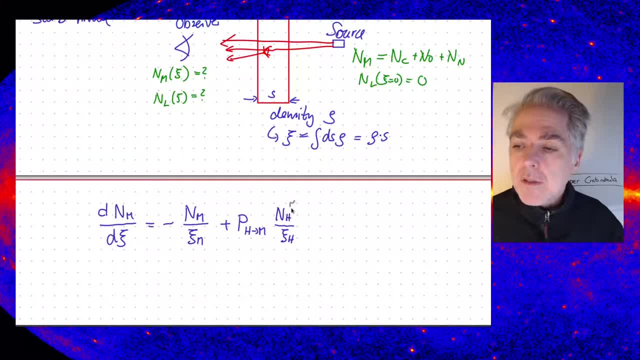 This term here, however, we want to neglect. So we basically say: this is: this is roughly 0, or it's smaller than nm, let me put it that way. so this is much, much smaller than nm divided by xi m. so so this, we can basically neglect this term here. 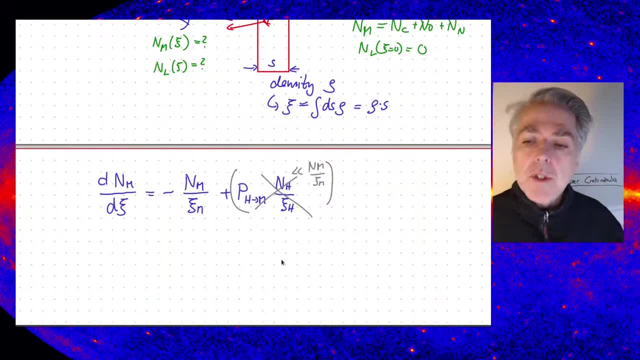 So we just take it out of the equation and then we would immediately be able to write down the solution for nm. Nm would be simply nm0 times e to the minus xi divided by xi m. so that's that simple, But while doing so, we will also. we also want to solve. 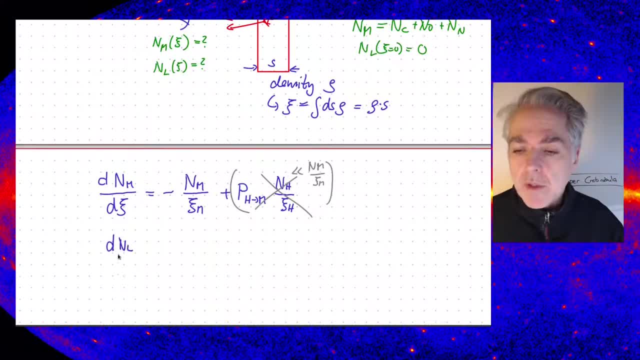 The equation for nl. so let's look at the equation for nl. That would be again the losses through spallation, that is, they light elements. they would also do spallation and they would produce hydrogen and helium. so there would be nl divided by xi l. 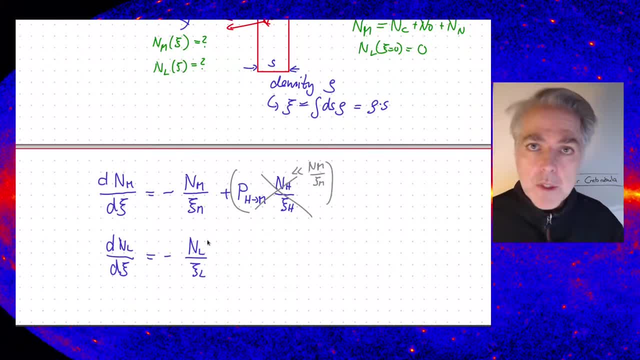 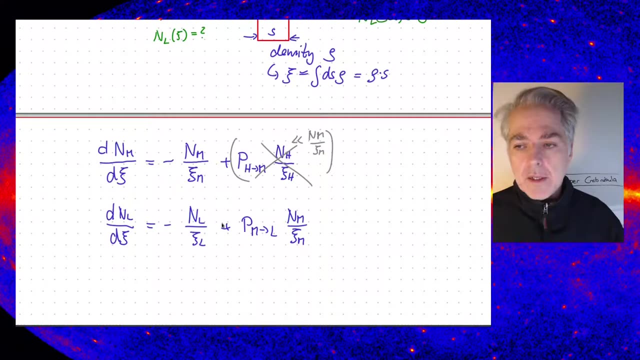 And we now have essentially the particles which are heavier, and the ones which we want to consider here are the medium mass group. so we would have here then a term which is medium: the probability To go to light times nm divided by xi m. so this is, these are two equations which are coupled. 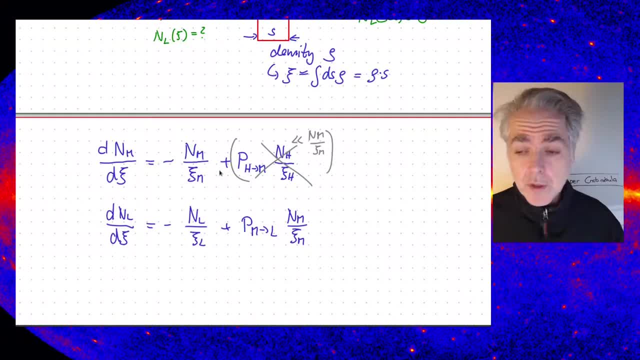 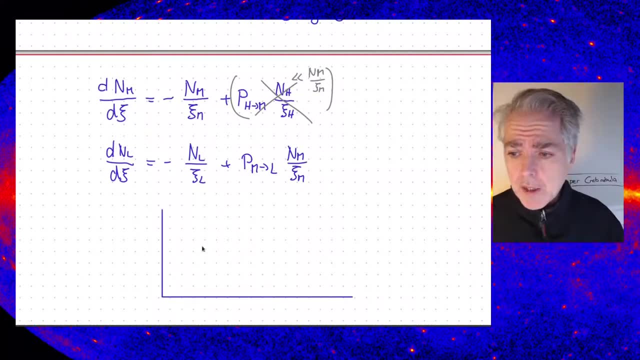 They are not too difficult to solve and for example, the long air book. you find the solution to this, but we can essentially just draw a graph to get at least now an understanding what will happen. so let's assume this is now the, the number of particles after some path length xi. 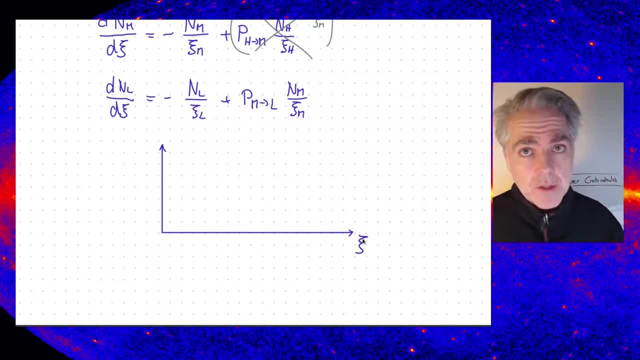 And xi is not known. we don't know. we don't know how thick the slab is, we don't know the density at a priori and we don't know the geometrical distance. so let's assume xi is just free. we don't know it, we want to infer it as a matter of fact. then we will have for nm. the solution is very. 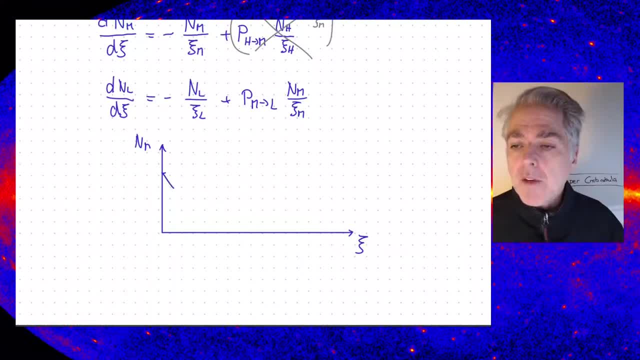 simple. so we start out with nm for xi zero and then we will have an exponential decay so that basically, after xi m we will go down to about one over three, so one over e of the number, and at the same time- Since this will feed this term here with some losses here- 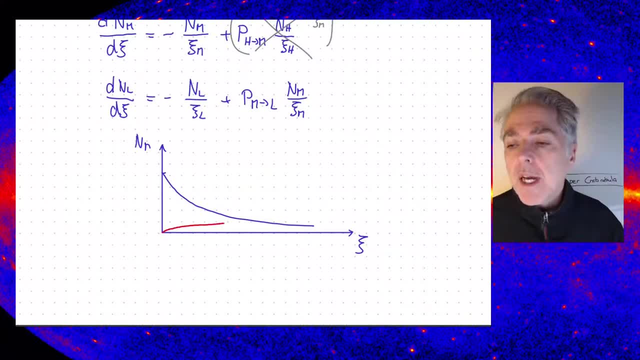 so we will have here some, some increase of the of the light particles, So it could actually go, even cross it through here, and we don't know now how far we are away. but now if we were able, so let me just write this down, this nl, if we are now able to measure the ratio of 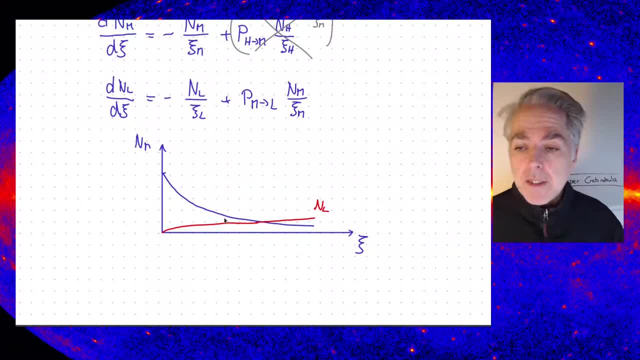 nm to nl. so we would fix that ratio. we would know that, for example, if it's like 0.25, and that's roughly what we get, we will be somewhere here. so then we would know what the xi is of our slab. and this is actually exactly what we do. 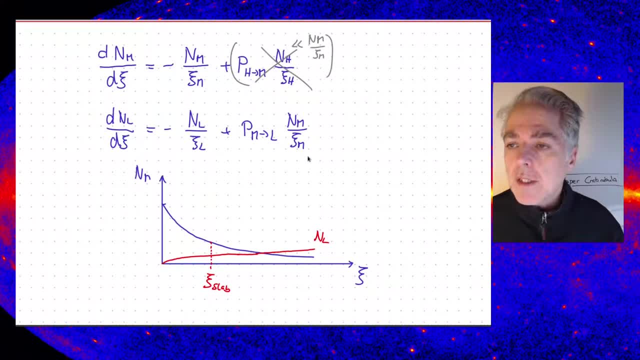 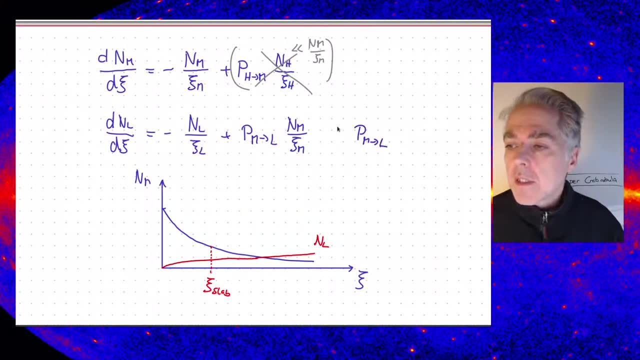 i'll let me just maybe also write down so that you know how to calculate this pml and so on. so pml can be selected accordingly. so I say that a ribo is given by is given by the ratio of the partial cross sections for producing lithium, beryllium and bor. 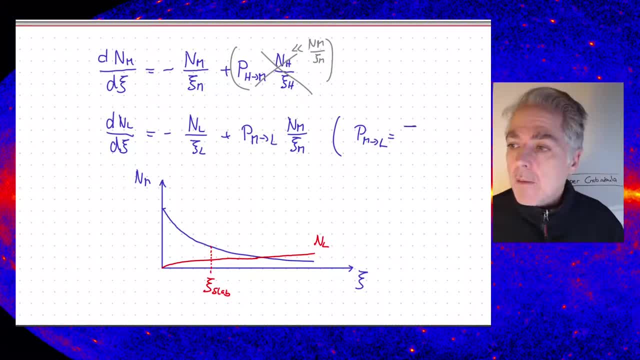 out of a, an interaction of carbon, nutrient, hydrogen and and and oxygen with the interstellar medium matter. so that would be for the light particles. let's make it maybe i, and i would be litium, beryllium and boron, and then over the total cross section for uh, for, for the, for the spellation, so including all other. 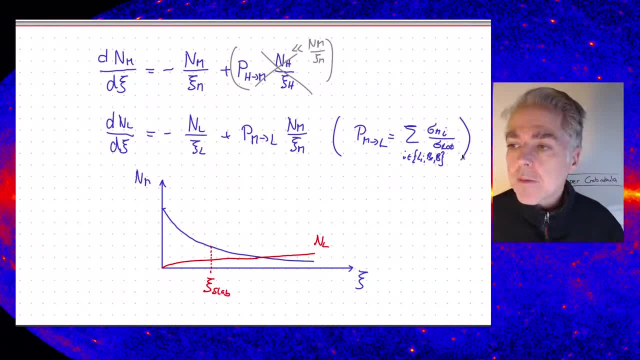 final states, including hydrogen and helium, for example, and the xi m. i should also say, for example, how you calculate this. so xi m, for example, is given by the cross section. so that's essentially just a row divided by the interstellar medium density number. density times the cross section. 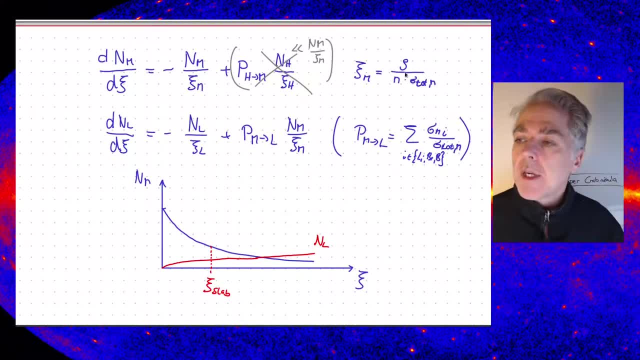 so this would be the total cross section for interacting with m and so n, n is the the number, density, density of the interstellar medium, and rho would be the mass density. and you can also rewrite it, because number density and mass density of course related by the mass number and the mass of the nucleon. so, um, we could basically now infer this this: 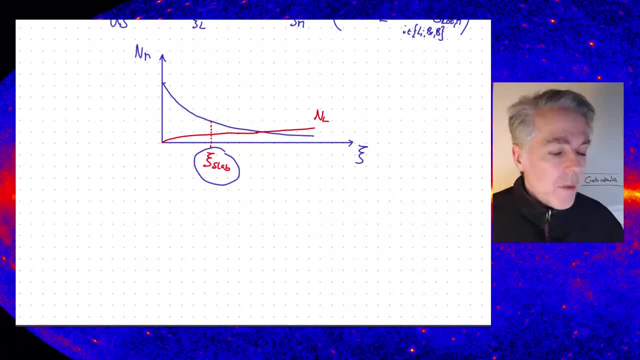 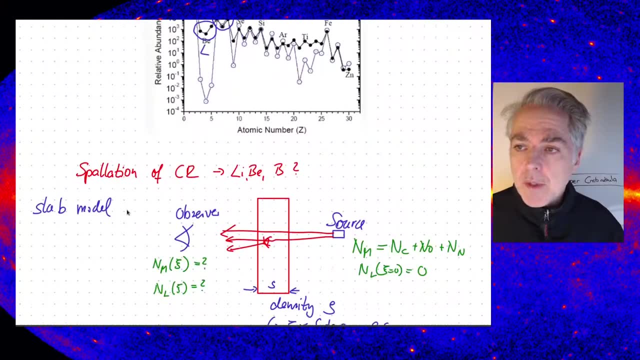 row slab by measuring it. but before we go into that, let's have a look at once more whether this, um, uh, these, these, these abundances that we see, keep in mind there's already some particular way that these abundances are grouped here, if you look at it. 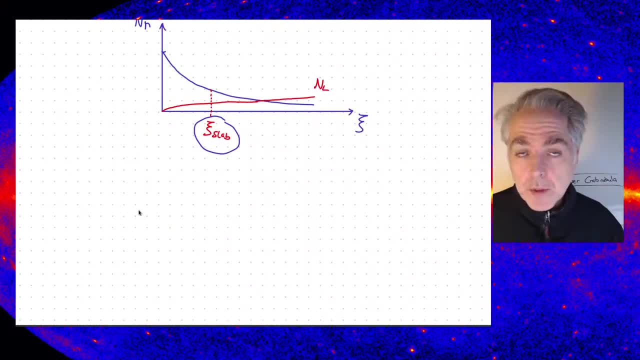 whether they relate maybe to the actual partial cross section to produce, for example, lithium, beryllium and boron. so i i looked them up for you. so we've got the cross section for any of the medium elements to become a lithium that is 24 millibar. 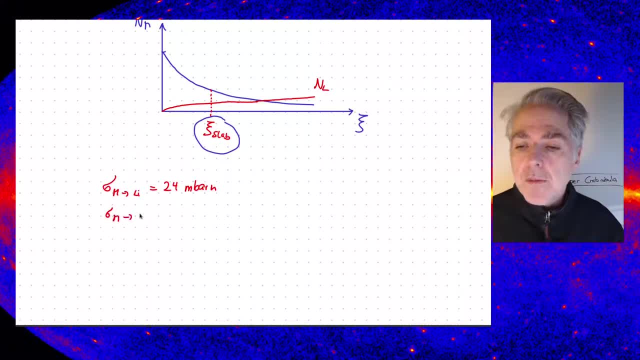 and the second margin of the nextworker. 15 millibar is about 50 millibar and we'll do a sixteen millibar and a passionateifier after that, by what we recall when we look at the two of the things that are going on in our 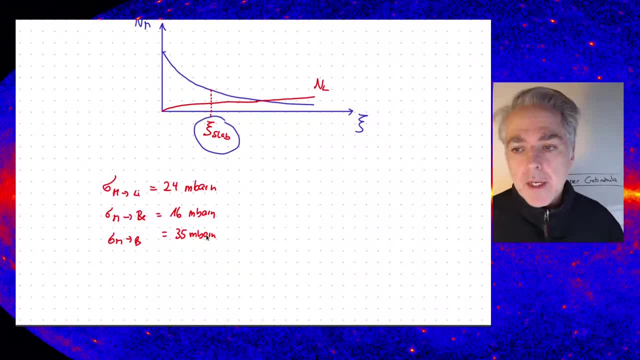 own logic in this section of grains, then you'll see that we see that the marine sources have fairly different diameters. amperes, apparently an actual will. some millimeters are much less than the linear sources and that's a side click capable of доступ to all the earlier Air andfeit can also react to eigentlich badly wise. 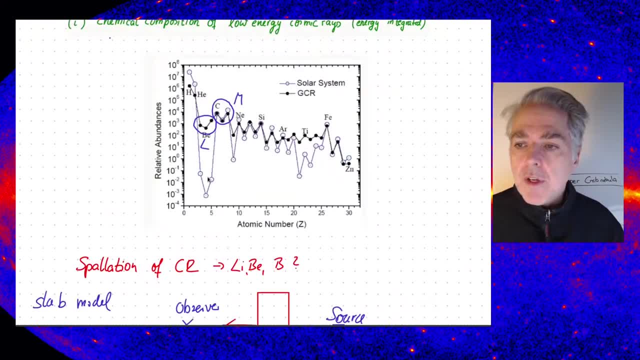 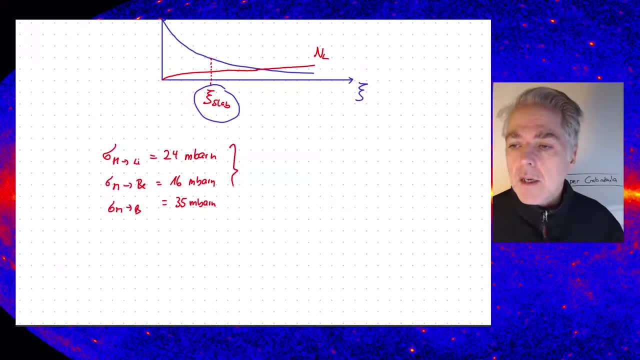 the large abundance you would expect for the, for the boron, and if you now look at this one, this is exactly what you have here. okay, so this is already quite good and this is consistent with the, with the abundances that we measure. so that's, that's good. that means that our spallation assumption, basically 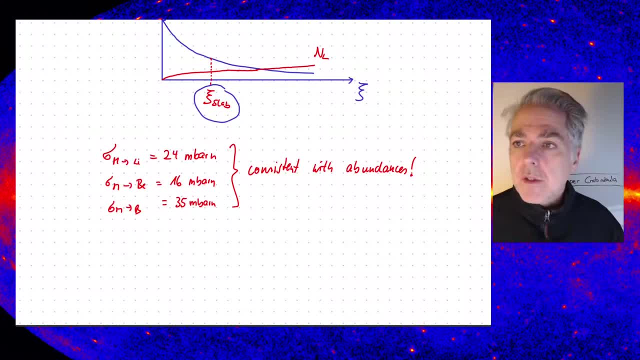 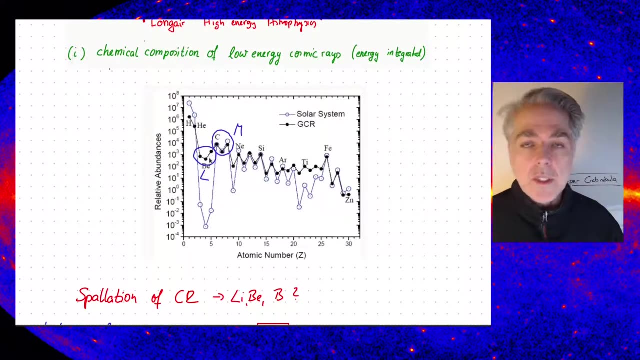 is consistent. now we measure. let me just conclude this one to you. so the nm over nl that we measure is about 25 percent. so this is essentially. you take this graph, you just sum those three ups and you sum those three up and you basically see it's about a quarter of of the, of the more massive ones. 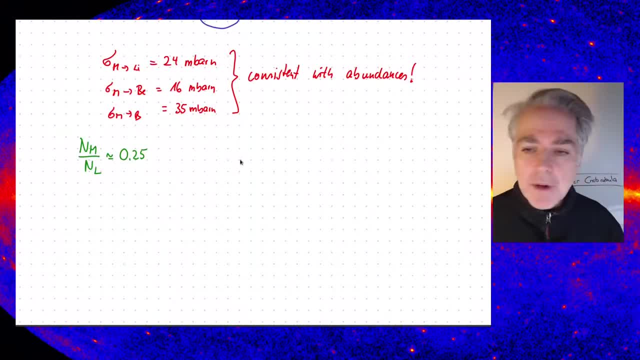 for the medium group. sorry, this should be the other way around. it's not nms, nl over nm, it's about 25 percent, and so you can then go to your solution, which i didn't derive here for you, but you can look it up, as i said, and then you can infer this slab distance. so this is an important number now. 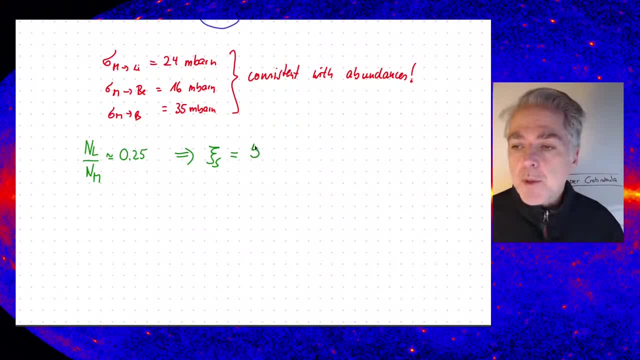 so it turns out. this is about it's slightly below five grams per square centimeters, so that seems to be rather small, right? but imagine you would measure a larger ratio. you would then get a larger value of this xis, and it also seems to be very small. 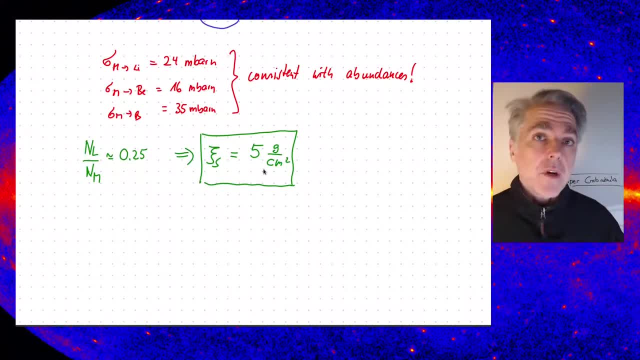 if you look at the graph here, you can see that the nm over nl is about 25 percent. if you compare that, for example, with the density of our atmosphere, so our atmosphere as such is a full column. density has more than a thousand grams per square centimeters and for a nucleus 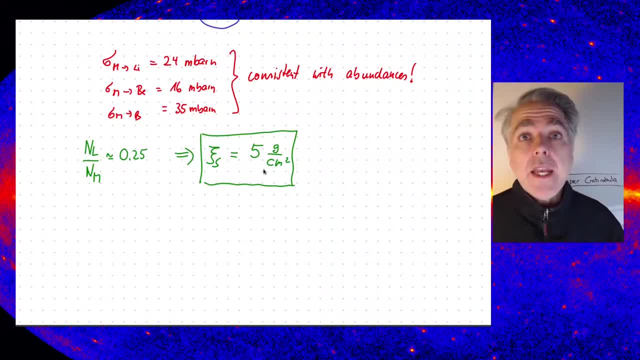 a cosmic ray particle passing through this slab? it will be, even though it's, you know, several light years, it would only pass through something like five grams per square centimeters. let's now make a rough estimate, assuming that the cosmic ray particle would be basically just traveling in. 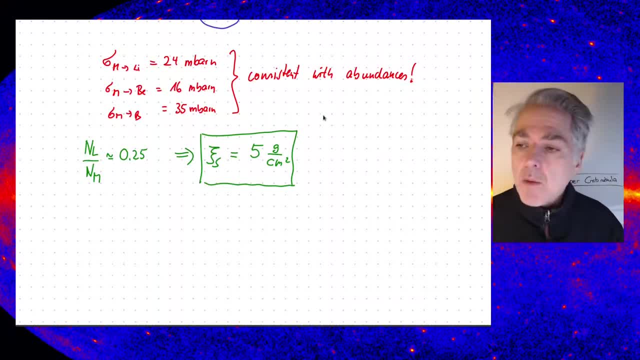 the galactic disk and not going outside of the disk, then we would say in the next year or so that the cosmic ray particle would be just traveling in the galactic disk and not going outside of the disk. the number density of the interstellar medium is about one per cubic centimeter, so it's easy to 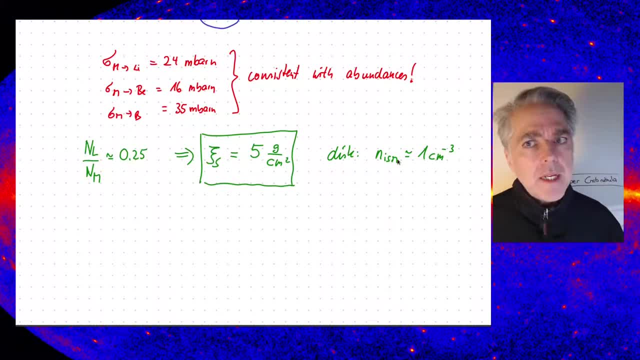 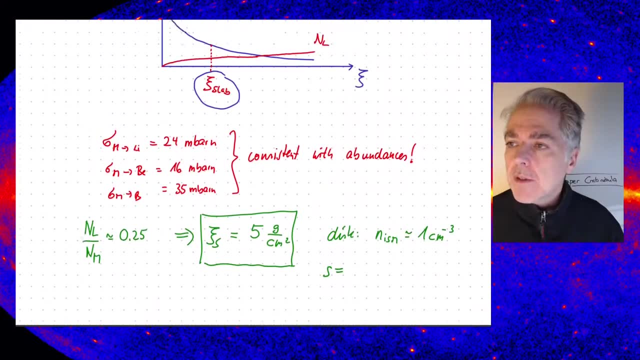 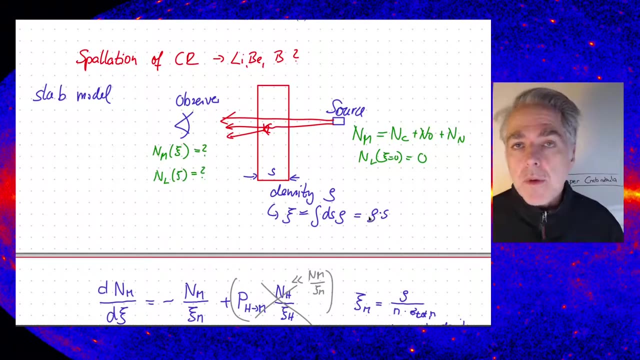 to remember. and so how much does that mean in terms of the path length? because we said remember, we said s would be. then you know, if we go back to the way that the xi is defined, so xi was defined as rho times s. so we know rho because we know it's roughly one hydrogen per cubic centimeter. 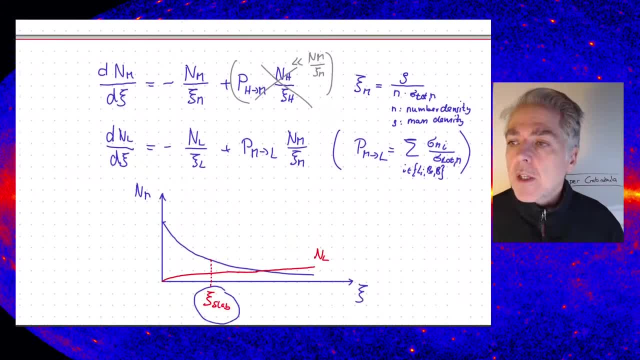 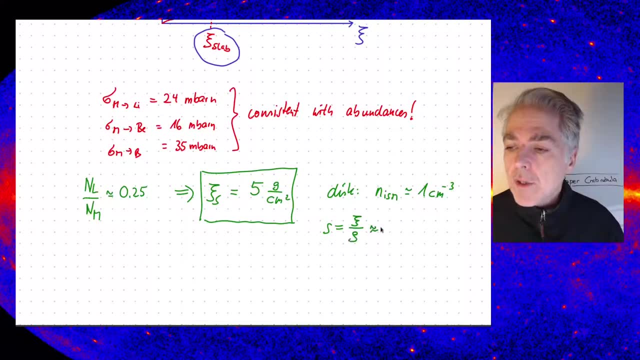 we know the xi to be five grams per square centimeters, so we know the x, i to be five grams per square centimeters. so let's have a look how large s is. actually s turns out to be. so that would be xi over rho, and that's of the order of about one mega parsec. so one mega parsec means ten to the sixth parsecs. 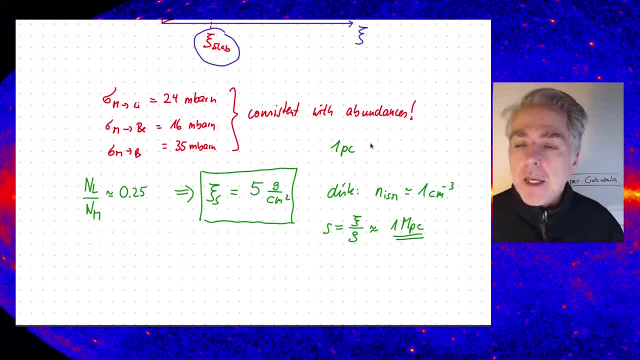 and one parsec. for those of you who don't have, maybe, uh any any um deeper astrophysics or haven't taken any astrophysics courses, one parsec is essentially a distance scale which comes from the fact that, uh, an object or a star which is about one parsec away. 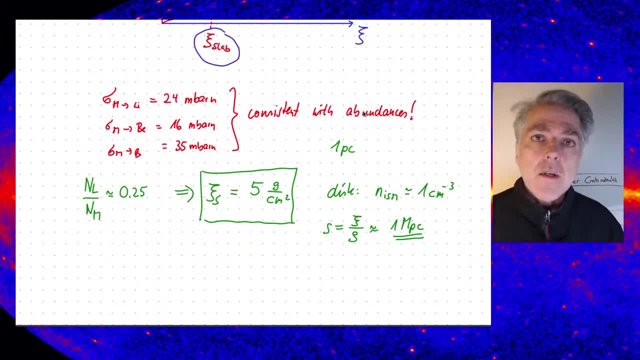 we would see as going through the um, uh, the, the motion of about one arc second in the sky because of the motion of the earth around the sun. so that's one arc second per year that we see this moving in the sky, and that corresponds to about three point, about three light years, that's 3.08. 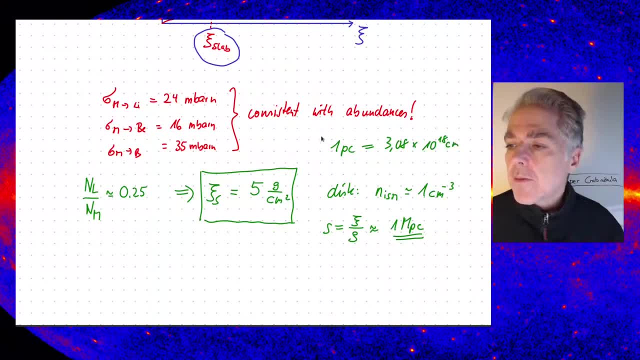 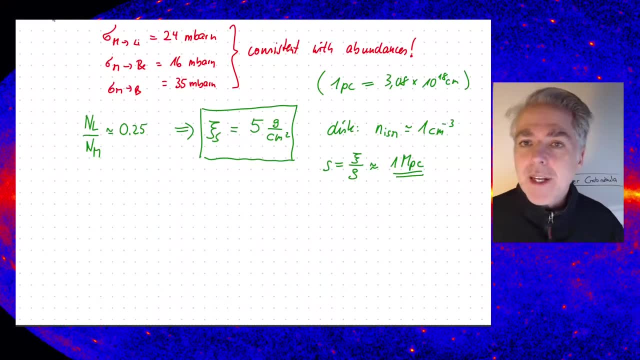 times 10 to the 18 centimeters and just to put that in perspective, our galaxy. to have a very simple model of our galaxy, maybe i just draw one here. so our galaxy is about this thick. that's the galactic disk and it has. it has a diameter of about 30 kiloparsecs. 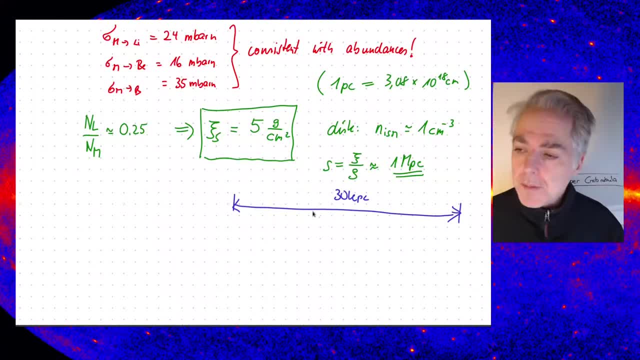 and has a thickness of a few, of a sort of 100 parsec or so. so that means that if the cosmic ray particles travel for a mega parsec distance, this is a much larger distance that they travel than the dimension of the galaxy. this means that the particles must be confined to the galaxy so they do not. 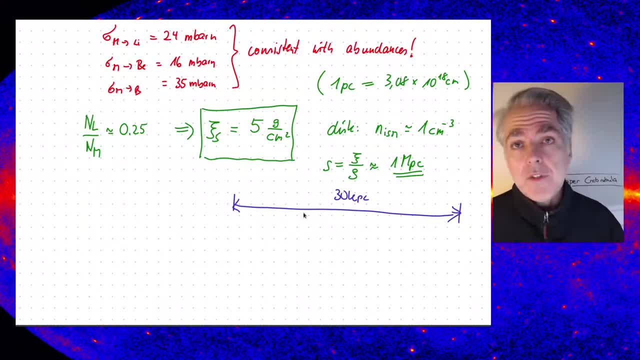 just travel freely and then just basically leave it after a path length of up to maybe tens of kiloparsecs, but they basically have to be going around and around and around several times, because this is much, much larger than the dimension of the of the galaxy. now there's two, uh, sort of 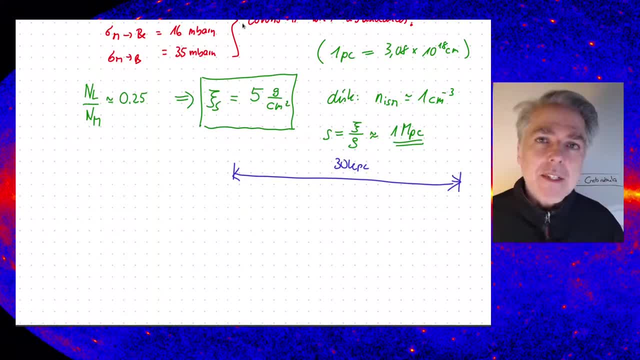 let's say of ways that we can use the earth to travel and to measure the distance of the galaxy, that people have been looking at this data and then come up with some suggestion how to model it. So the one is the ad hoc assumption, which is so-called the leaky box. 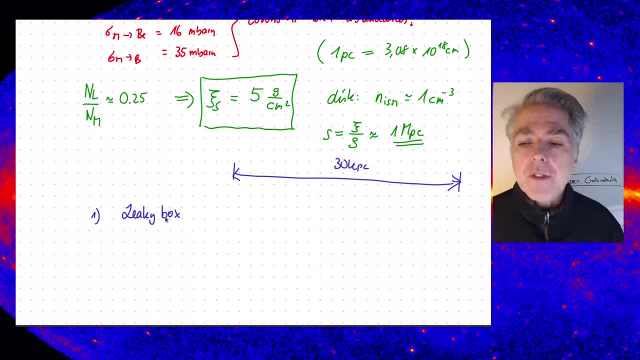 You'll find this in the literature still floating around this term, and it has some, let's say, good points to it. So the leaky box is essentially similar to our one-slap model in unphysical assumption, So we cannot just have a slab, as I said. 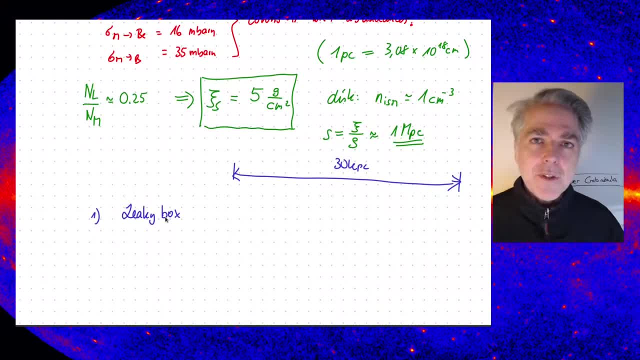 because the particles would basically, depending upon the distance of the source towards us, they would just pass several different distances of the slab, and this would be then the average would be 5 grams per square centimeter. However, since the slab must be bigger than the galaxy, 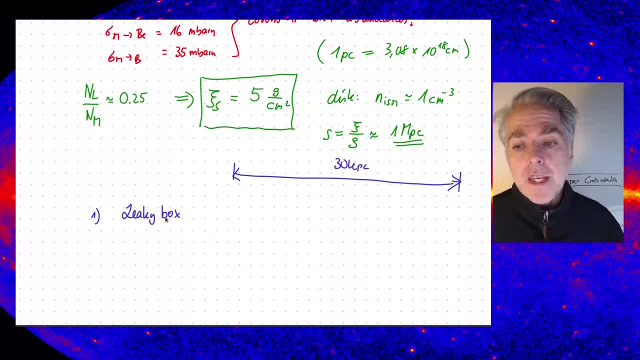 this cannot work. So the next way that people have been looking at this, when you go from the one-slap model, so maybe I'll just put this here. So the one-slap model does not work, obviously because the galaxy is much bigger than the slab. 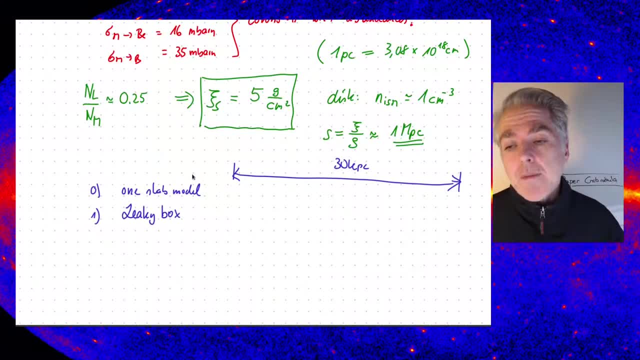 Sorry, the galaxy is much, much smaller than the slab would have to be, So the leaky box essentially assumes that the particles move freely and, however, they are confined to a box, So the moment they hit the boundary of the box, 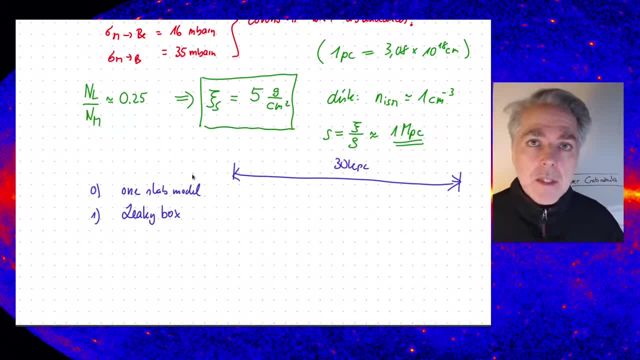 they get reflected and then they basically bounce around in this box until they have a small probability to leave the galaxy. So each reflection has a probability of whatever very close to unity. but if it goes through several of these reflections, at some point they will leak out. 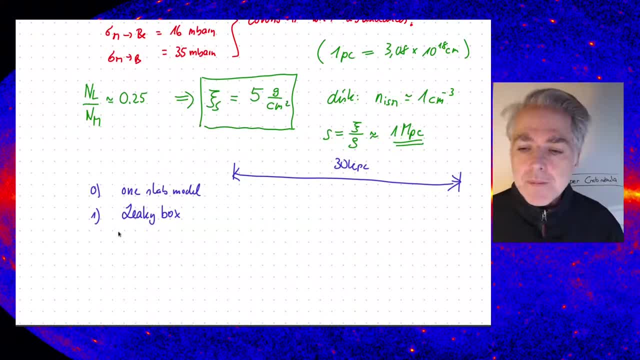 So this is sort of the next stage step of the one-slap model, but they're both unphysical because our galaxy doesn't really have a boundary where things could deflect off. So they're sort of ad hoc models, but they help to put some kind of model into perspective. 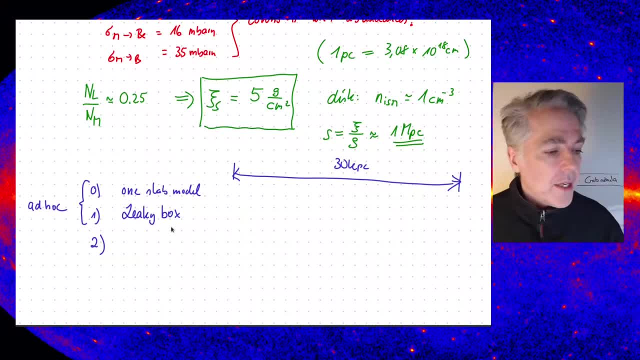 Now the more physical approach is to say that we have a diffusion zone and maybe also some convection of cosmic rays in the space, In the galaxy And the cosmic rays. they would not bounce around, but they would basically move, like, for example: 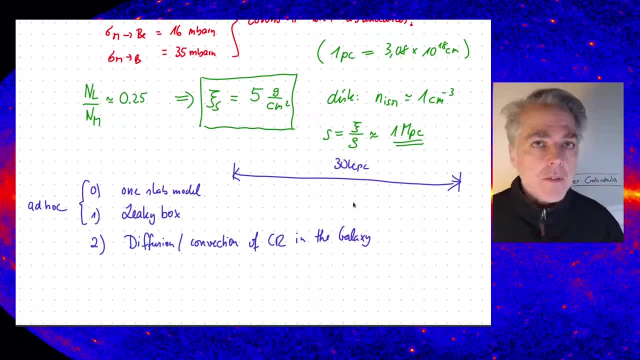 as you know, a gas, when it expands, or when you have something expanding or moving in our system like an atmosphere, you find that this moves diffusively. or if you think about charge carriers moving in solid states and so on, there's a diffusion process mostly. 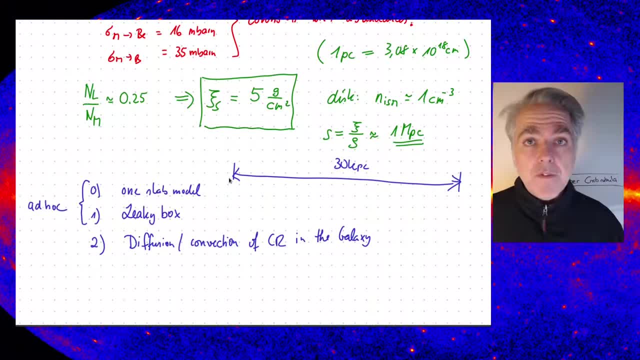 So a diffusion process requires, however, that the mean free path length must be very small, And this is something we will discuss a little bit later, but it's a very important thing. But the process would be such that, as the sources inject cosmic rays, 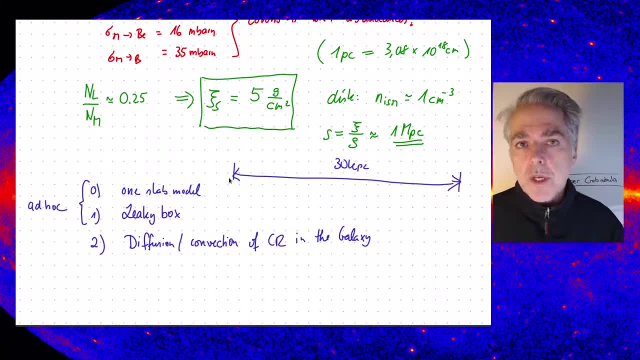 and they would move diffusively And in some regions where you have some bulk motion of the interstellar medium you would also have some convection maybe, but mostly it's moving through diffusion. And then you would essentially if you start diffusing out of the galaxy. 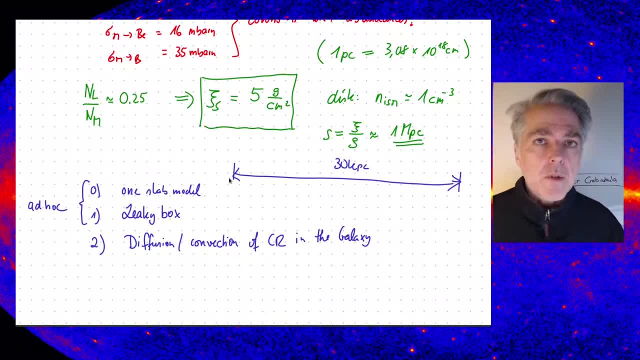 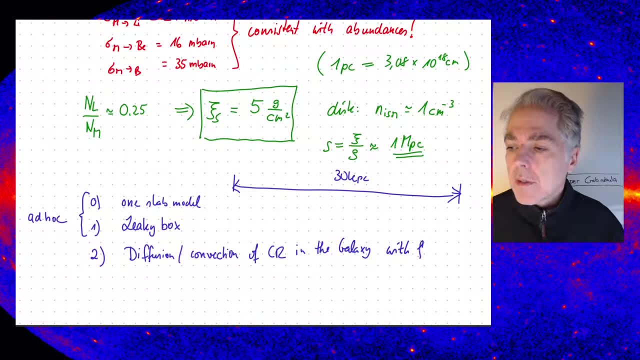 at some point out of the galaxy, these particles would become free and they would not diffuse anymore. So there would be some free escape at boundary, And that's sort of the most physical model that people are using these days. Now let's talk a little bit about this diffusion process. 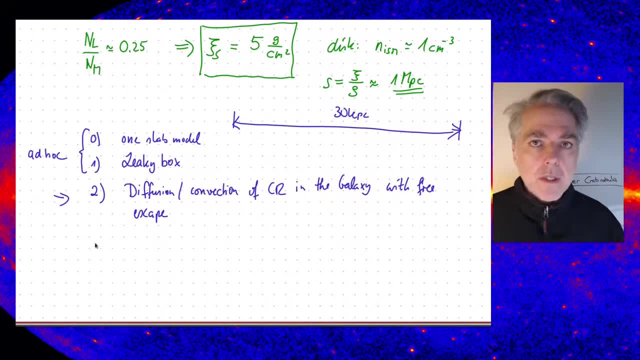 so we understand what the characteristics are. And let me just remind you about diffusion, as you have learned it in physics in your bachelor's time. So diffusion has this funny mechanism: whereas the particles are bound in a medium, in a way that they basically have a very short path length. 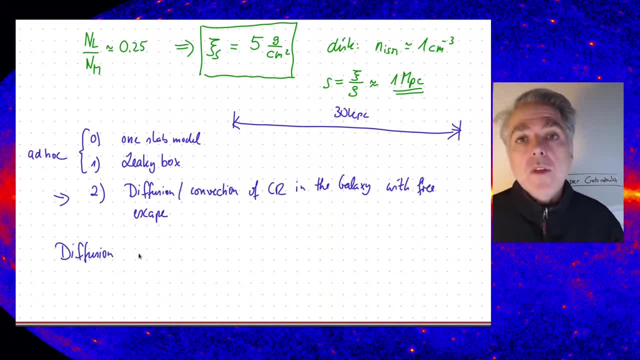 and then they bounce back and forth. So since they bounce in a random way, the average distance they travel is zero, because they get scattered backwards and forwards So they don't really have an average displacement, but the average distance squared that a particle would diffuse out from. 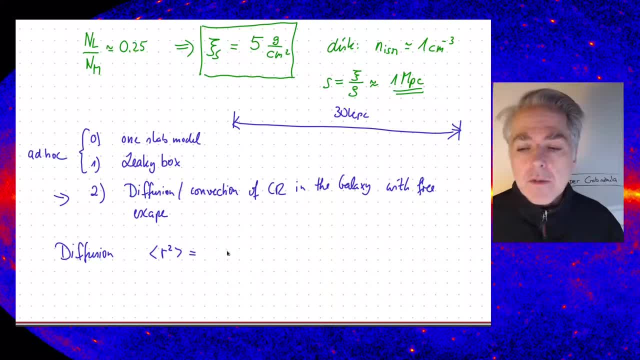 let's say some central point increases. So you know, imagine you start out with a singular particle distribution and after some time, later, the particle distribution would spread out in space. It would still have, on average, the position zero, but the squared value will be non-zero. 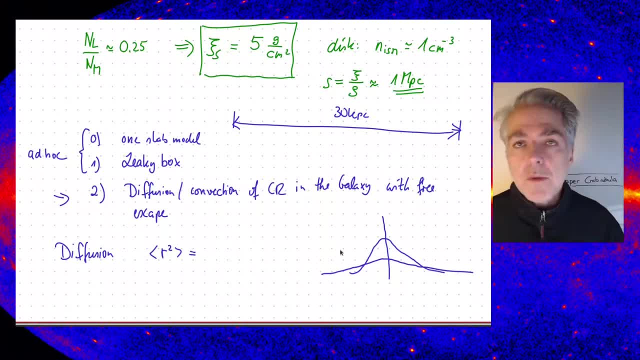 And this would basically, you know, diffuse out like this, and so on and so forth. So it would basically smear out And this is what happens. So diffusion has this property. that r squared goes with d times t, where d is the. 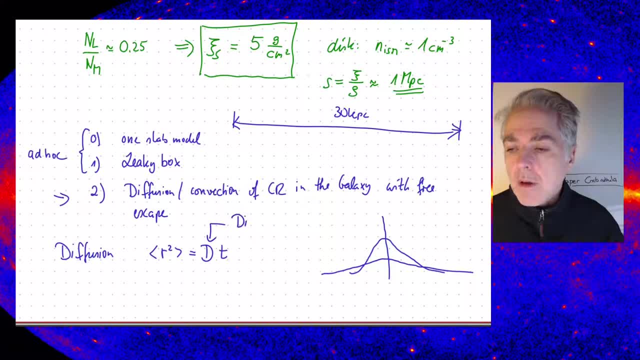 the so-called diffusion constant. It has the properties of square centimeters or length squared over time. And the diffusion coefficient has also physical meaning because it's tied to the mean free path length. So d is given by the mean free path length lambda between two scattering points. 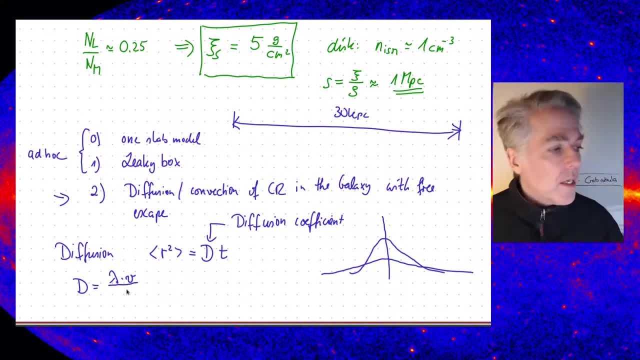 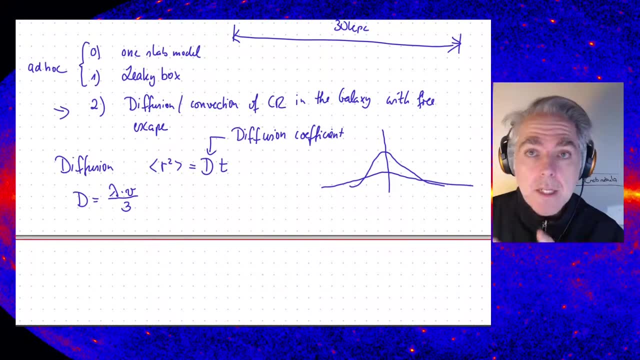 times the velocity with which a particle move around divided by three. So we have to think about what it could be the mean free path length in the case of a collisionless particle. In our case, the only thing which happens to cause a deflection of the cosmic rays 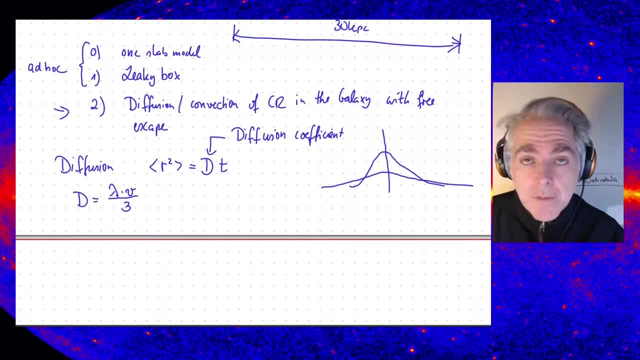 is the magnetic field. So we don't know the magnetic field, but we can assume that this is the dominating or the smallest path over which a deflection occurs, given that there's no collisions over galactic scales. So so what we therefore assume is that lambda. 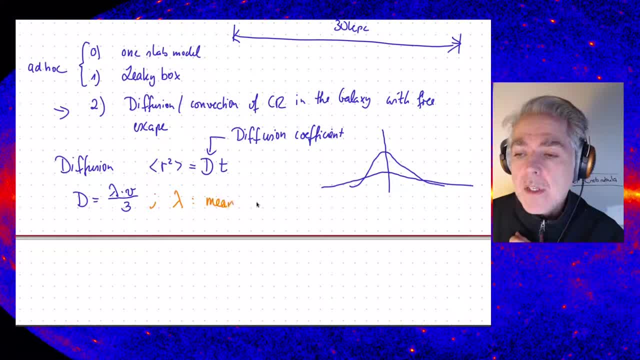 is the mean free path, which, in the case of diffusion, corresponds to the path distance over which the particle gets deflected substantially. And so we assume this is equal or similar. equal to the to the gyro radius. And how big is the gyro radius? 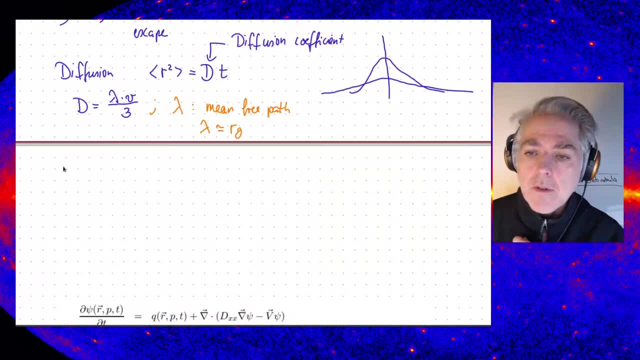 Let's write that down for a moment here. So the gyro radius is given by the momentum perpendicular to the B field, Divided by the charge, divided by the magnetic field, And as an example we can say, or as a number: 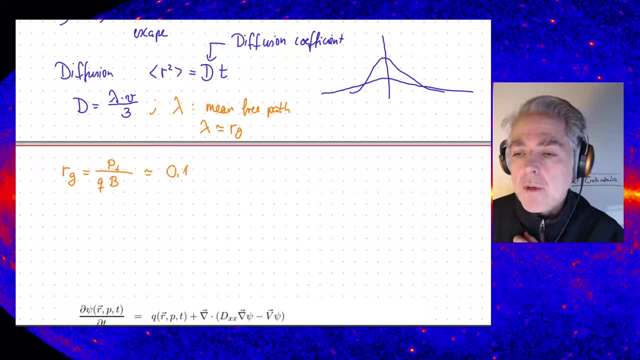 so that you have an idea how big that is. So the gyro radius is about 0.1 parsecs. for charge equals one, So that shall be the charge number of the particle times for an energy of the particle. I write this now in energy, not the momentum. 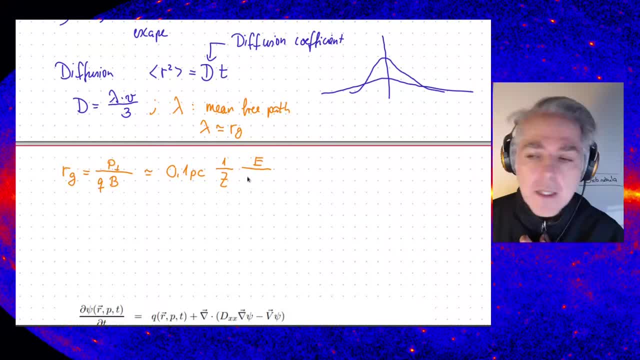 but they're equal for any realistic purposes of energies that we're looking at, For 10 to the 14 electron volts and for a magnetic field of on micro gauss. So one gauss is 10 to the minus four Tesla. so this would be 10 to the minus 10 Tesla. 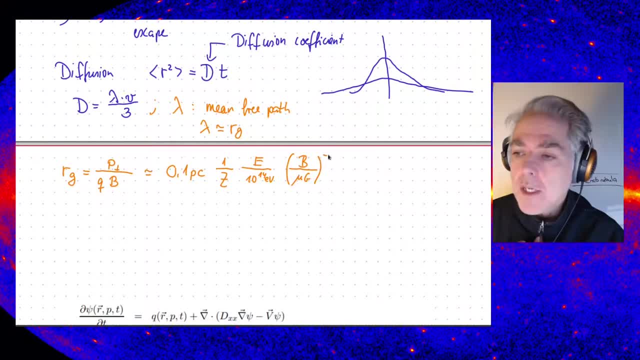 But in astrophysics we often use the Gaussian system, so that's why I also use it here. So this is obviously much, much smaller than the collision length scale for one particle per cubic centimeter. So that's really really much, much shorter. 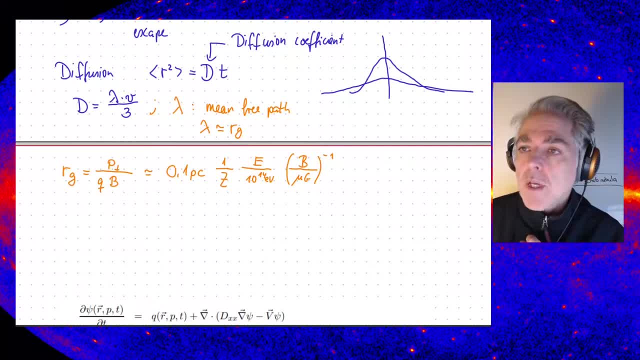 Therefore, this is the one which is most important. So let's see how that basically tells us about particles, and then we'll go on to the next slide. So let's see how that basically tells us about particles. densities as a function of time. 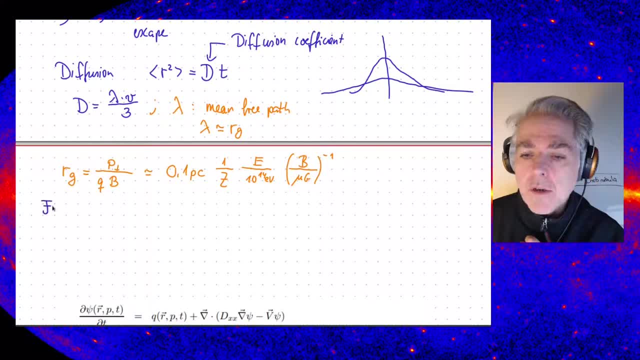 So there we have this well-known law that came up by this Dr Fick. He basically said that a current of particles, a current density of particles, is proportional to the gradient of the particle number, density, and it goes with minus D. so diffusion coefficient again. 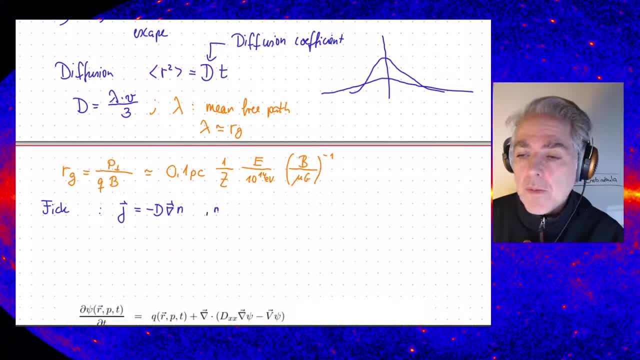 And also if you have mass conservation, so this is the mass density and also the number density and this is the flux density. So mass conservation or particle conservation, I should say not mass, it's really particle conservation. but okay, they are equivalent of course. 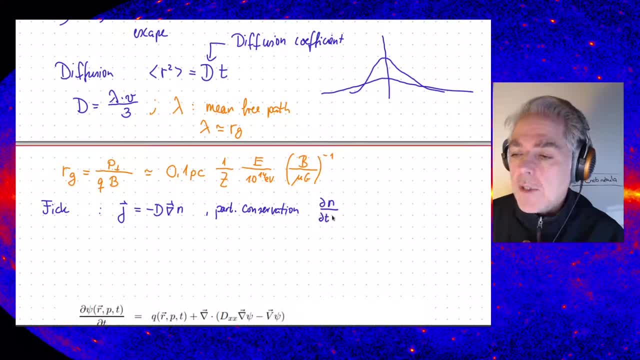 So particles do not get destroyed. So you get: Dn over Dt is equal to minus gradient of J or divergence of J, and if you combine these two you basically get an equation which says Dn over Dt. so basically now I replace the number density. 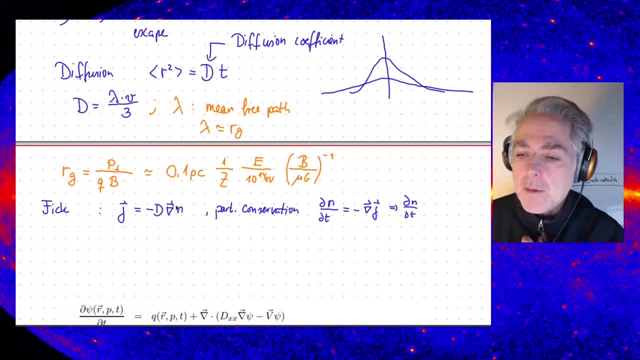 or the flow density, with minus the gradient of N. So Dn over Dt is then divergence of D times gradient of N, And this is in the case that you do not have any particle losses. We know that there's particle losses. there's losses due to spallation. and there's maybe other losses that we have to consider. and there's losses due to spallation and there's maybe other losses that we have to consider and there's losses due to spallation and there's losses due to spallation. 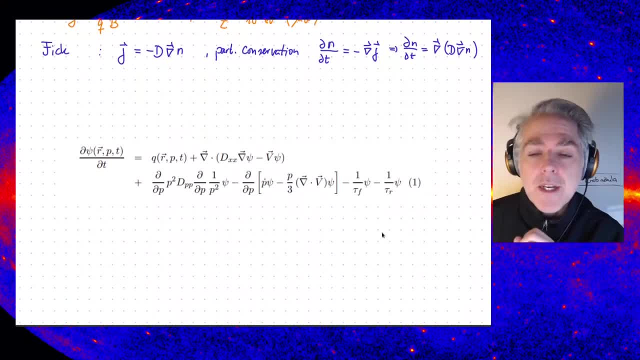 so the full equation that you can write down. I just put it here. So if psi is the number density, I took this equation straight from the 2007 review article. so that's the number density, which is a function of the spatial coordinate r. 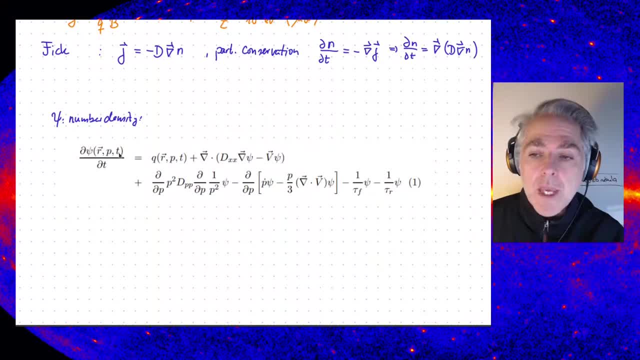 so function of the form momentum p, and it's a function of time. so you find this is the term that we just looked at. so that's, dxx is the spatial diffusion coefficient. Note: it's written here with two indices, so basically you can also allow this to be anisotropic. 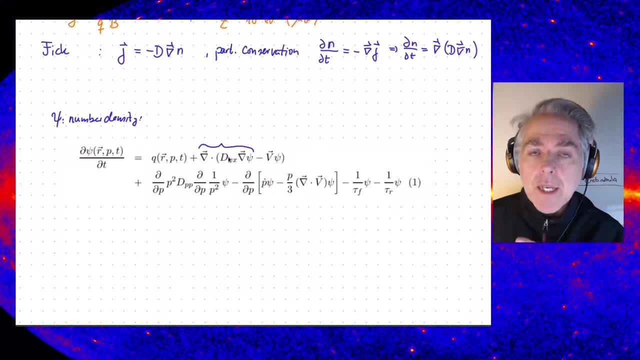 so this could be depending upon the direction, and this is very likely the case if you have structured magnetic field. So this diffusion, and then we have here convection. I didn't go through that before, but convection basically means the medium has a bulk velocity of v. 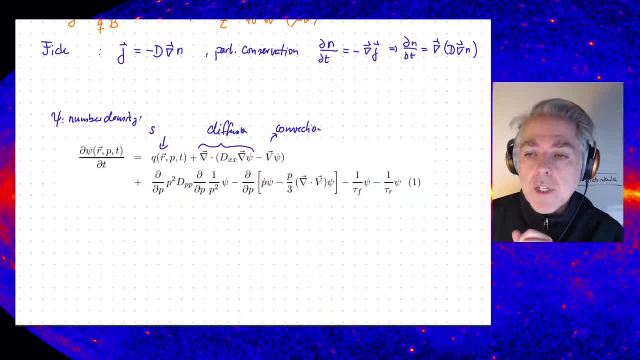 The q which is put in here. that's the source function. so that would be anything which creates, accelerates, cosmic rays. Then we've got another term here which has this dpp in it and that's similar to spatial diffusion. 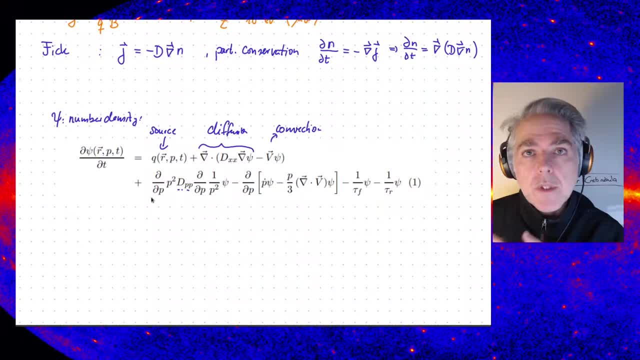 You also have diffusion in momentum space, so that could be any processes which lead to acceleration or re-acceleration of cosmic rays. So that's diffusion in momentum space. And then we've got terms here which are also continuous. so you basically have 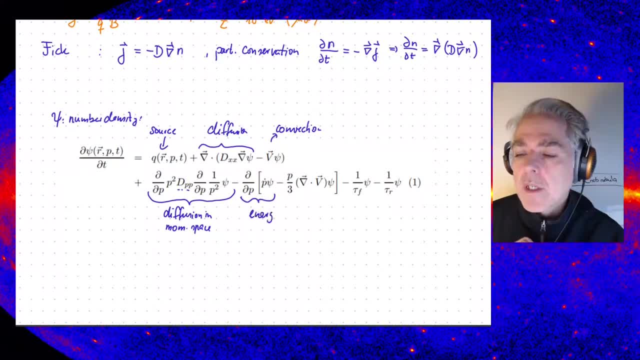 a continuous energy loss term Could actually also be a energy gain term, so p dot could be positive or negative. And then you've got one more term which has to do with getting with the bulk velocity, and that's basically adiabatic losses. 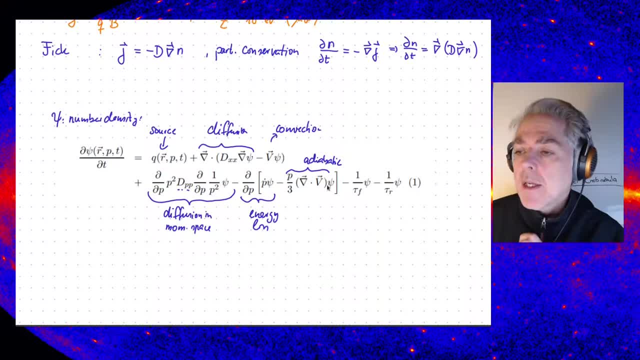 So you have to lose some internal energy when you expand the material. And then we've got here two terms which look very similar to what we had before, but instead of xi we have the time here, because this is now written down as a function of the time. 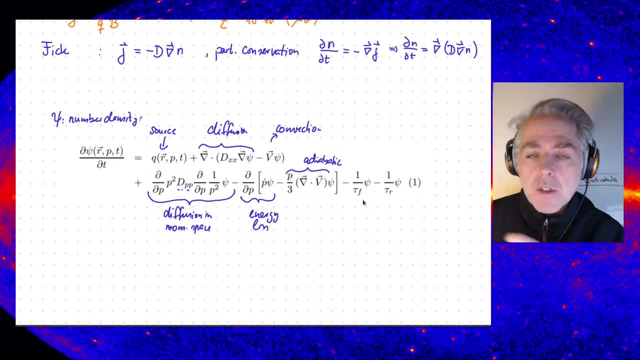 And so we've got one which has to do with fission, so spallation. This basically removes particles with some time constant, and this one also removes particle. that's basically radiative decay. So that's actually the equation which describes the whole process of cosmic ray. 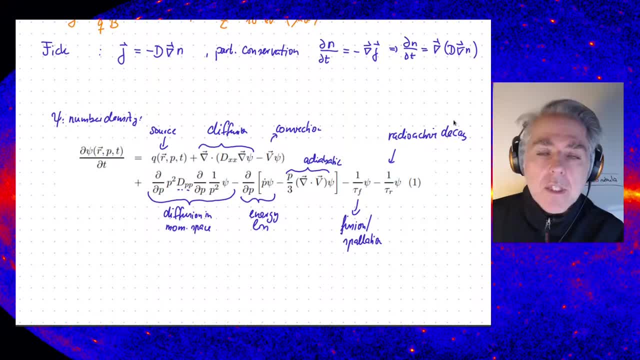 propagating in our galaxy and, you can see, solve this equation, albeit only numerically. There's not really a simple way to do it And the physics that you have to put in can be quite complex, in a sense that the diffusion coefficient, for example, is not a number that you can basically write down the way I did it now. 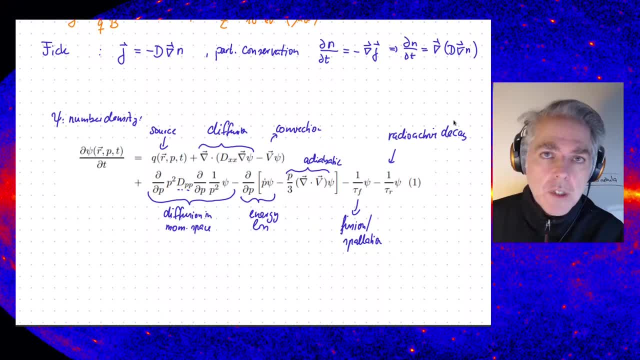 because it depends upon the B-field structure. So the diffusion coefficient is actually quite a complicated function. It could be also anisotropic, as I said. Energy losses, for example, do not really continuous. energy losses do not play a big role for the hydronic component. 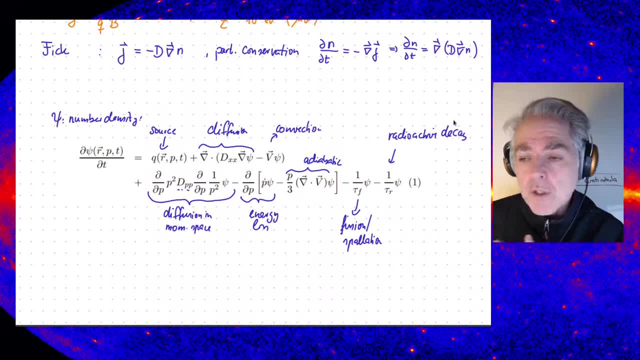 because they basically always do first any kind of fission or processes. Adiabatic losses only play a role if you have a rapid expansion, So this is usually not so important. And also convection terms. they sort of compete here with the diffusion terms, But for energetic particles. 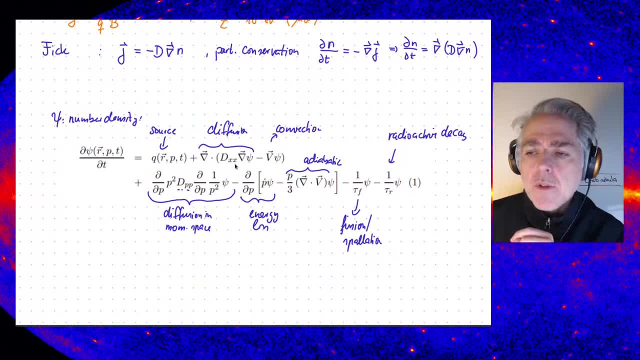 it's the diffusion term which dominates, because the diffusion coefficient is usually energy dependent and will grow with energy, with some power, And whereas the velocity is just something which is a constant term. So this will be dominating at large energy. This will be for small, energy is relevant And this is not relevant. So, and also the diffusion in 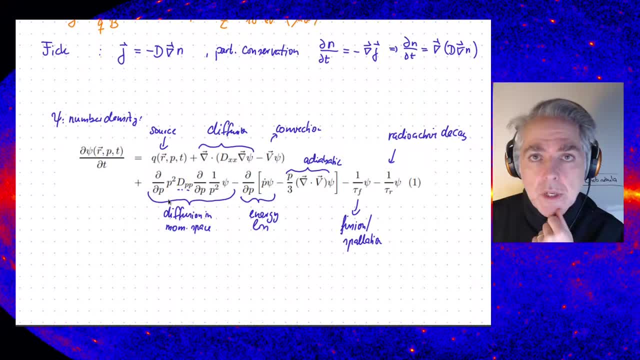 momentum space is often enough neglected because it doesn't really play an important role, And so you can bring this equation in a simpler form And then you can solve it also in this, in the way that we discussed it. Now, after we looked at this equation, which is tough to solve, but we're not- 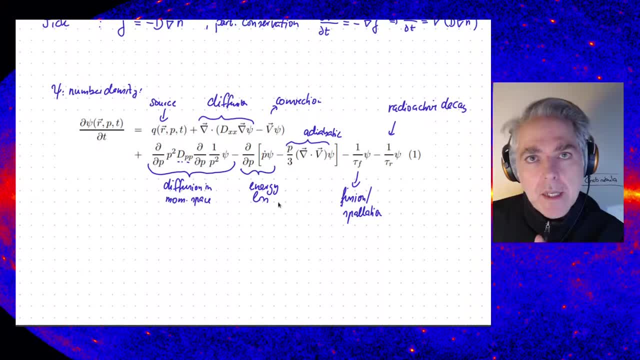 going to attempt to solve it, But we can still, as I said, use some of the very simplified models to get an understanding of what's happening. Now let's look at the data. What does data tell us? So one thing that we can infer from this equation is: you do this. 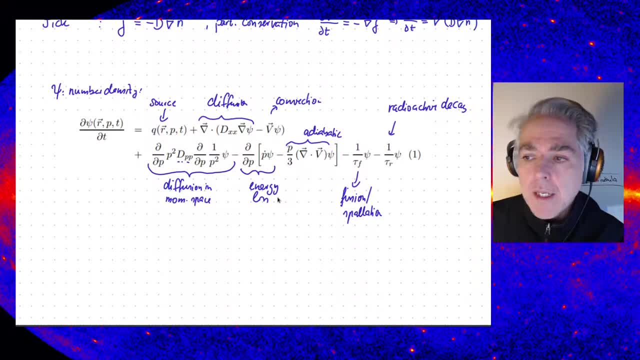 solution for the heavy particles and for the light particles, And you can basically do the same thing as we did in this lab model, a bit more sophisticated, And then you can predict secondary to primary ratio, like, for example, boron to carbon, which are the most abundant ones that you find. So this is turns out to be energy. 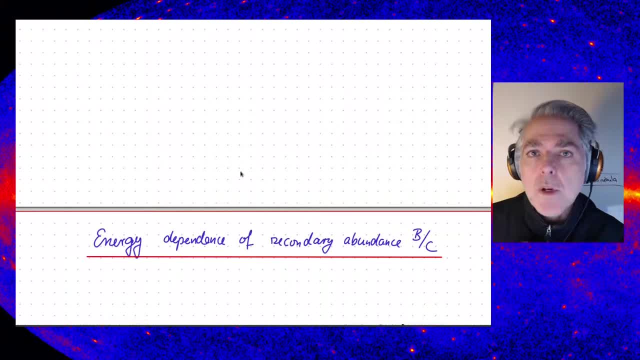 dependent. So it doesn't. it's not a constant number. The number I quoted before, 0.25, is again the integrated number, integrating with the whole energy range and also taking the three light species in some combined way. However, what you usually find in the literature is the boron to carbon ratio, because 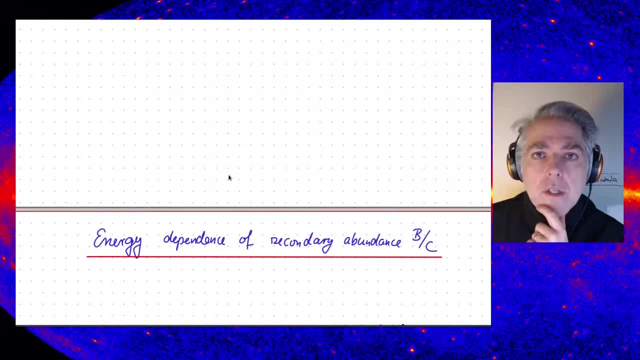 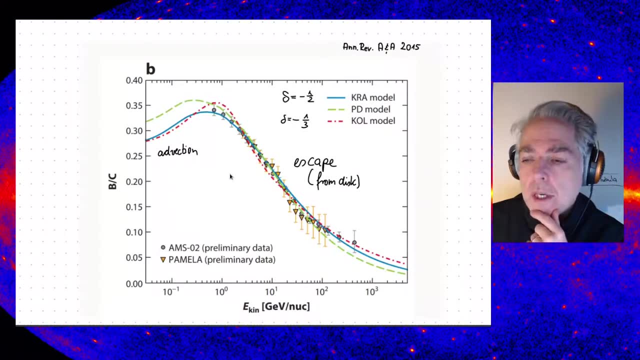 that's the one which is having the largest, the largest value, And so here I give you now something which is a couple of years old. Now, that's a summary of this measurement. Measurements that I quote here are the ones from the AMS experiment. So that's the gray points which you find here all along, And also the 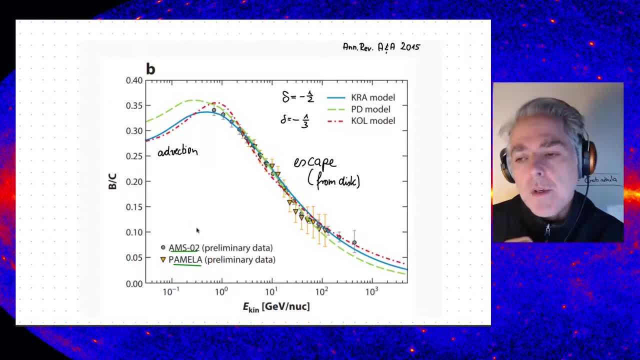 Pamela data. It's called preliminary data because 2015,. that was just preliminary data. But I like this figure because it has some also some models in it. And now let's look first at the qualitative way that this, this ratio, looks like. So you find that in the beginning it starts rising, So you 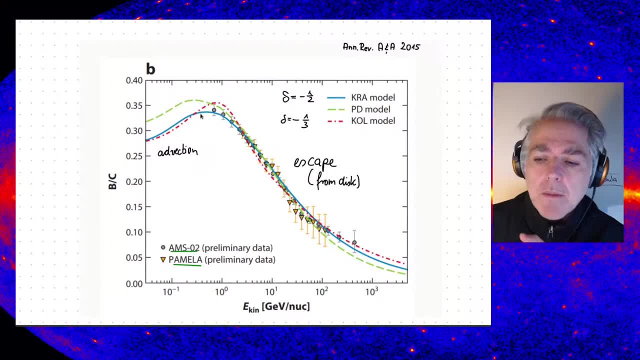 know the model start rising. I have to say There is actually some measurements Which go to the smaller values, which are below a GeV per nucleus, And there you find that they turn down again. this is not so easy to see, but the data really. 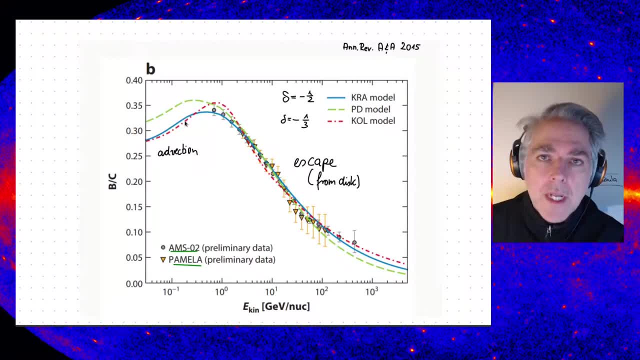 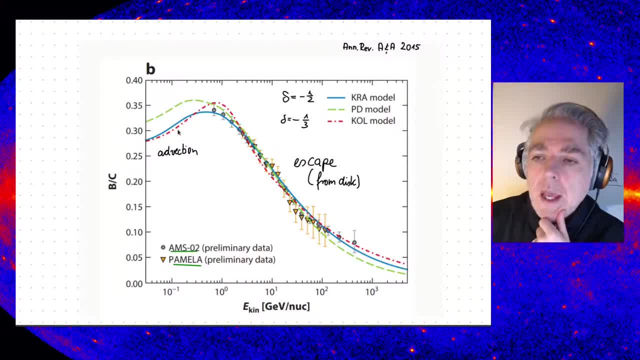 basically, at some point it falls back. However, this, this effective motion, leads to some depletion of cosmic rays at low energies. That's why you see some some drop off there. However, let's look at the energy dependence beyond that peak. there you find that the data follows pretty much a power law. So note: this is a linear scale on the the y. 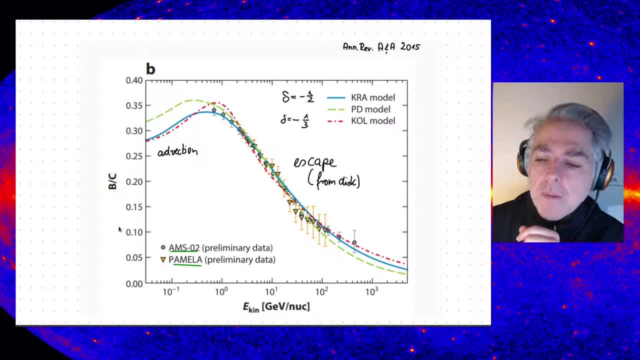 axis, So this gives you the value of B over C And there's a logarithmic scale on the x axis, So a pure power law. basically looks like some of these lines which are indicated to you And you find there's there's three models given here. I don't want to go into the details, But they do have a dominant difference, that is, they: 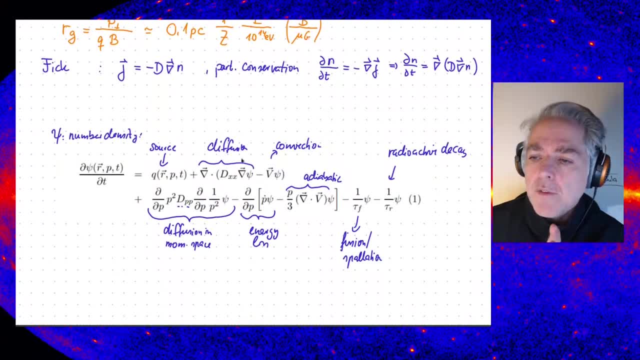 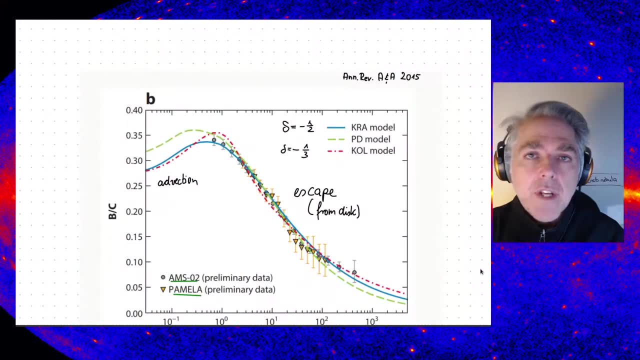 predict different energy dependencies of this diffusion coefficient that is used for this modeling. So- and this relates again to the way that the magnetic field looks like, not particular strength, but more it's the way that it has, let's say, spatial dependence. So what you can do is you can look at the so called power. 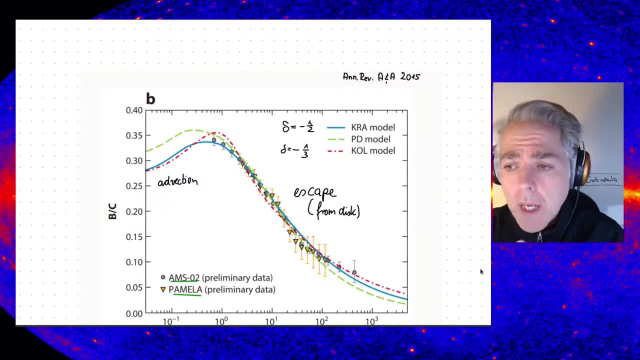 spectrum of the magnetic field energy density, And this one has then a particular power law index which depends upon the dynamical motion of the material. Interstellar medium is a highly turbulent medium, And therefore you expect that the turbulent flow will also reflect the power. 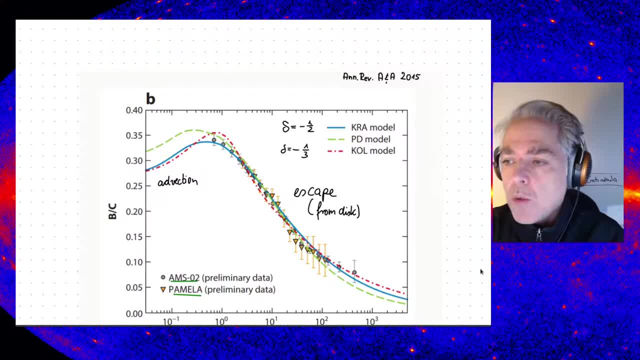 spectrum of the magnetic field, And there's two very prominent ways that this power law spectrum in the magnetic field energy would depend upon the wave number. So the one is the and the other one is a Kolmogorov, And they lead again then to different energy dependence of the diffusion coefficient, And that has to do with the fact that 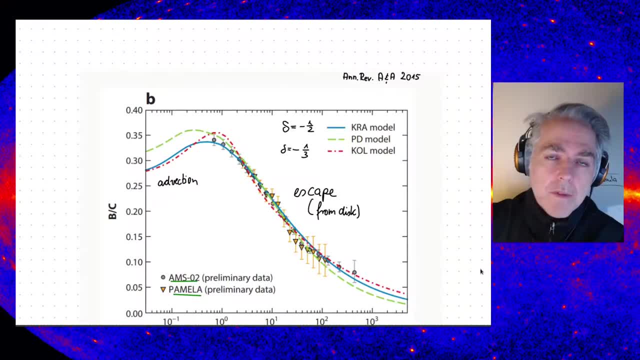 This is not just one homogeneous B-field, but the B-field is basically following such a turbulent scaling law And so, depending upon the energy of the particle or the energy of the nucleus, you will have a particular gyroradius, And if that gyroradius matches the wave, the inverse of the wave number of your power spectrum. 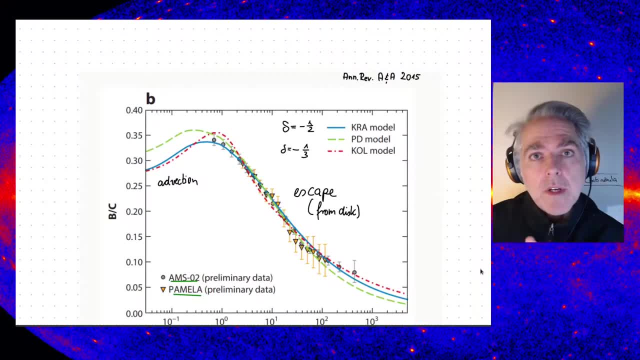 then you have some resonant effect which basically leads to maximum scattering of the nuclei, And this then leads to a particular way that this rigidity-dependent diffusion coefficient behaves. So there's the so-called Kreichnern power law spectrum and the Kolmogorov. 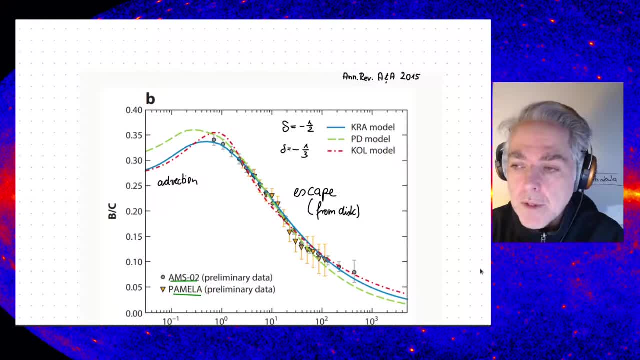 Kreichnern is going in the blue line with d to the minus 1.5, whereas the Kolmogorov- it's the red line- goes with d to the one-third. So now if you look at the data it's sort of not completely clear which one is favored. 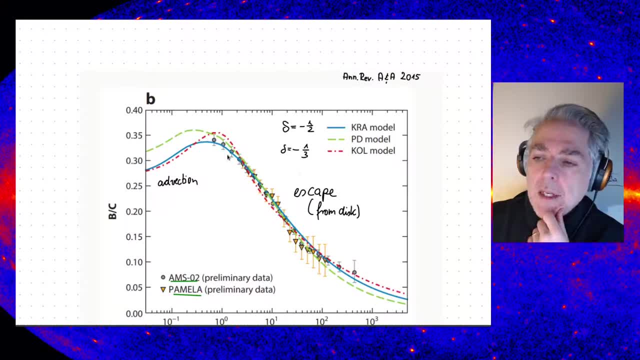 There's also another one which I'm not going to discuss, and it's the PD model, And it seems like that maybe the Kreichnern model is slightly better at describing the data than, for example, the Kolmogorov. 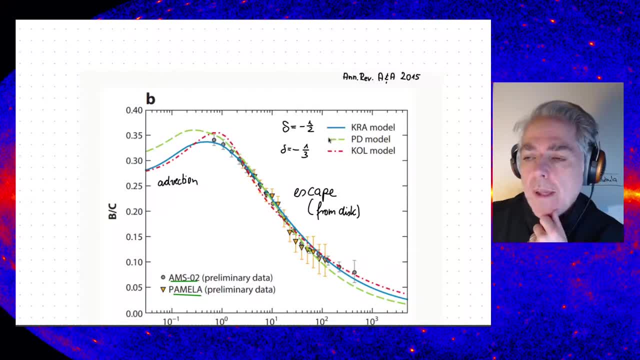 which has a slightly different slope here, And so this tells us a lot about the magnetic field structure. but this is not something I want to discuss in great detail here. But what we can basically make out there is that the diffusion coefficient increases with energy. 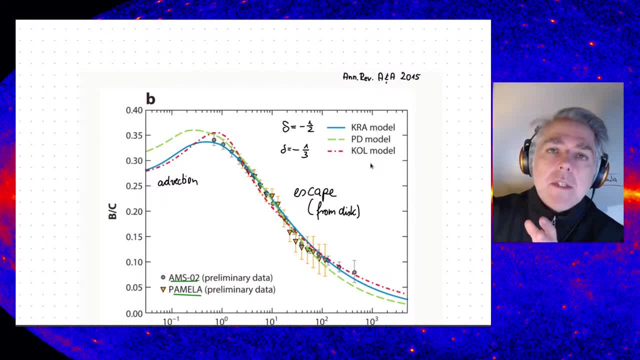 That means that the average square distance over which the particles can travel goes up proportional to the square root of d, And therefore the particles can travel further outside of the galactic disk, And once they start leaving the galactic disk they do see then a smaller magnetic field. 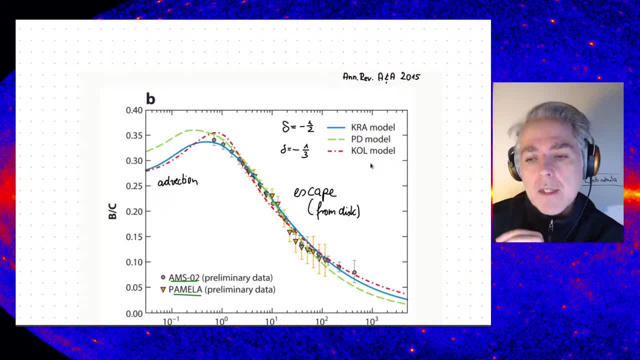 and at some point they can freely escape. So what we're seeing here in this b over c ratio is that particles with increasing energy will have a different if you go back to the one-slap model. they will have different slabs over which they traverse. 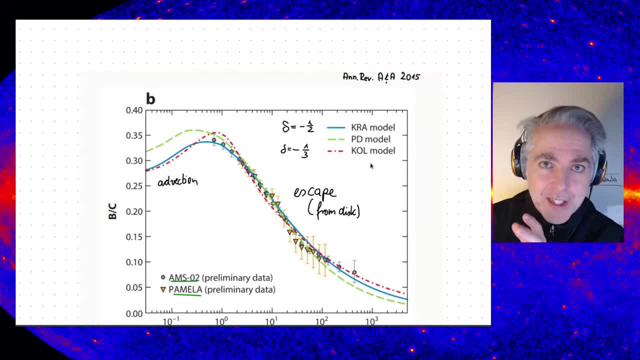 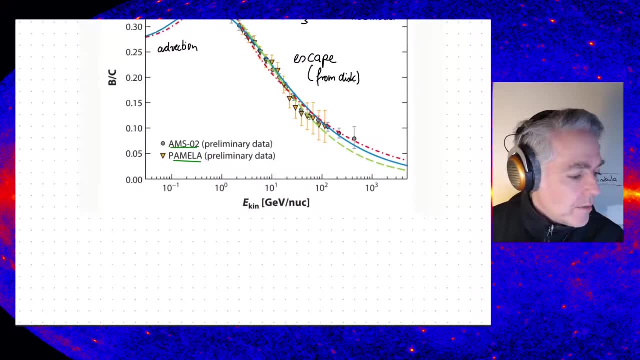 So there's a sort of energy dependence of the slab that is predicted through this diffusion. So we can also look at it in this very simplified way. So let's assume we basically say that we not only have the interaction but also escape. 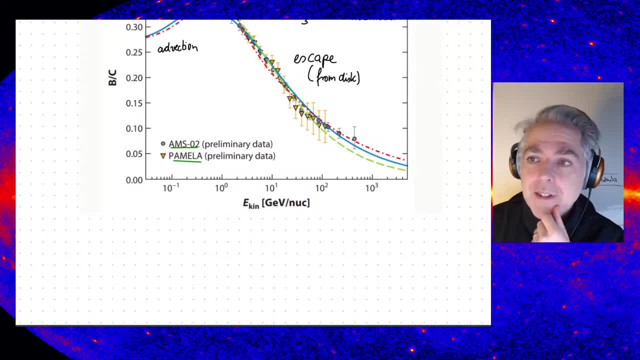 And then we can put our little equation up again. that is the one-slap model, but now we assume that the escape slab, there's a particular slab length which corresponds to the escape of particles. So then our equation basically comes back to: 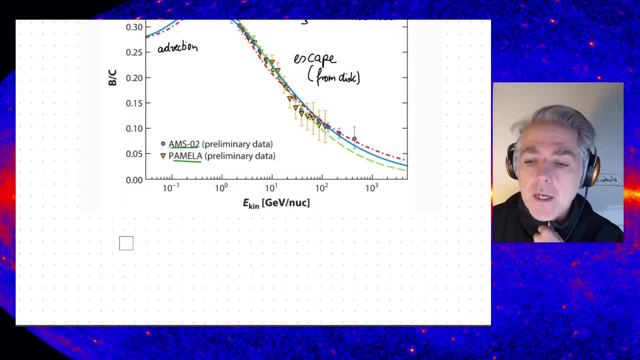 Oops, this is not So good. So that would be, then, our equation for the medium particles. So we would have PmL and Nm over Ξm- This is the term that we had for the light particles. 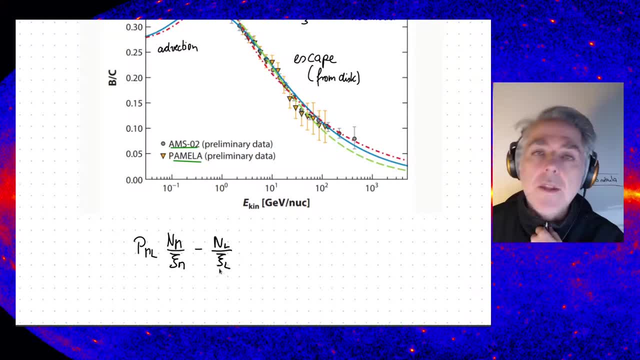 Minus Nl over Ξl. that would be the interaction losses of spallation. And now we add another term to this. That means that Nl is also depleted by escape. We call that Ξe, And that's supposedly now energy-dependent. 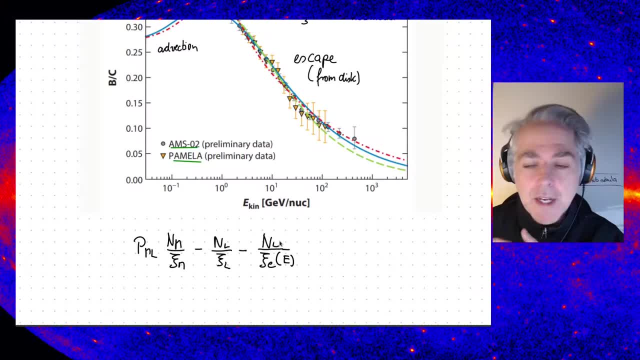 So even in our one-slap model we can just ad hoc say there's an energy-dependent escape length And that would be zero. And then basically, So I put it to be zero because now we assume that things are in equilibrium. 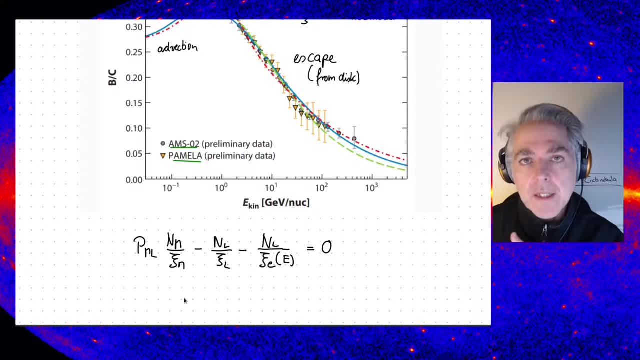 So that is not DnL over DΞ, but we say: it doesn't change anymore over time, So it remains constant. And if we now assume that At this part Over here, Over here, Over here, obviously escape becomes dominant, because you don't produce much boron anyway anymore, 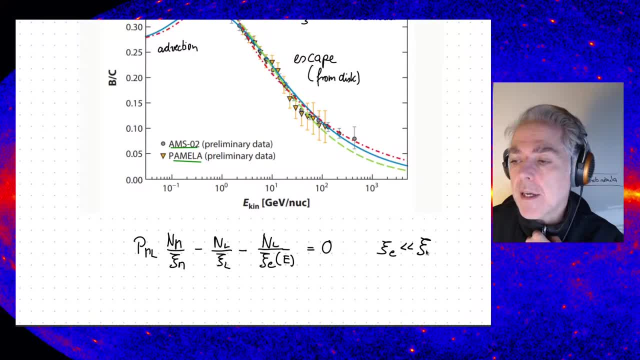 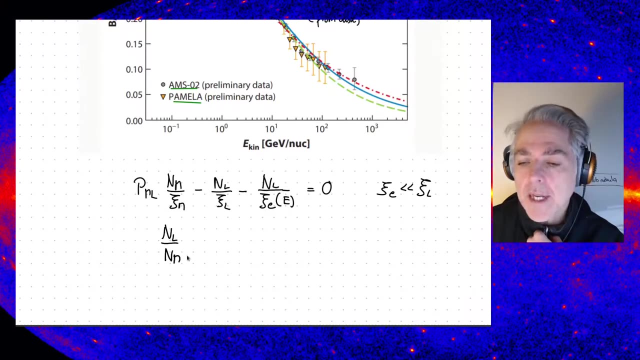 So the escape must be much smaller than Ξl or Ξm- And this is true for a buff- let's say 10 GeV. Then we can solve this equation again. in the same way We can calculate Nm. 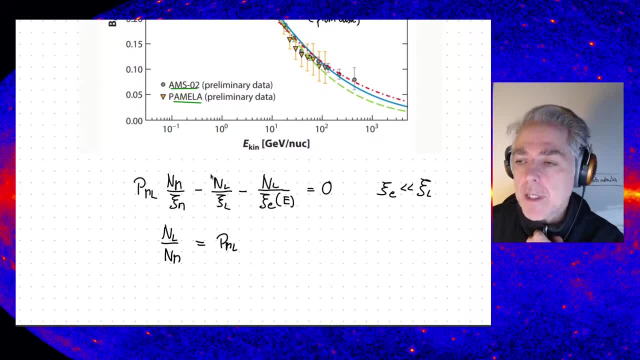 And that would be then PmL. You know, this term basically can be neglected. Then we have just this equation solving over here. So the Nm and the Nl, we can calculate the ratio. Then we've got PmL times Ξe, which is energy-dependent, divided by Ξm.